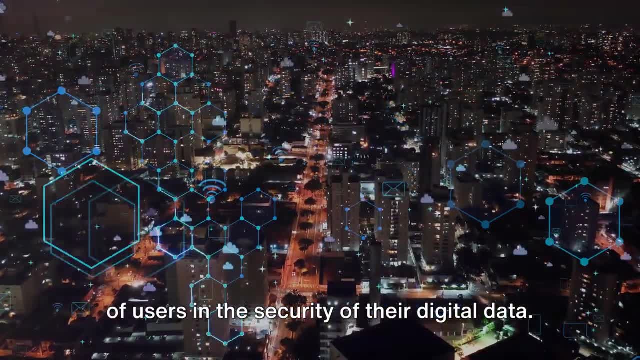 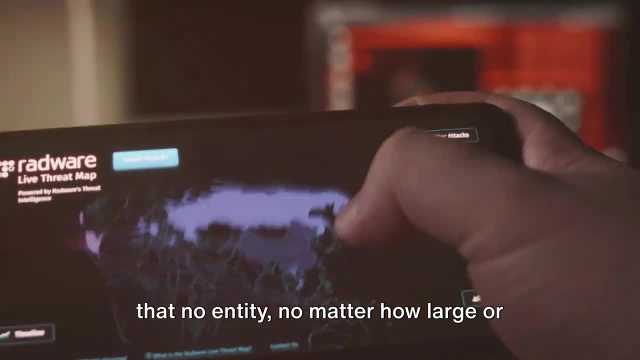 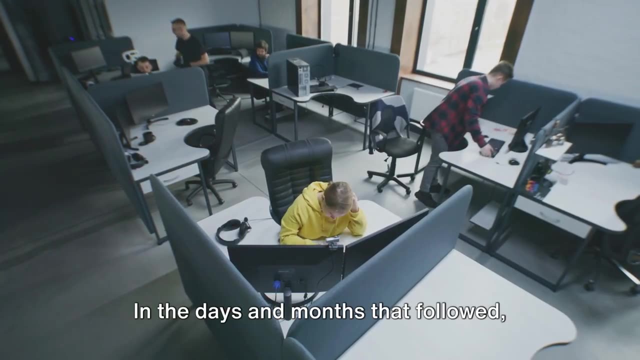 shaking the trust of millions of users in the security of their digital data. The incident served as a stark reminder that no entity, no matter how large or technologically advanced, is immune to the devastating effects of a buffer overflow attack. In the days and months that followed, Microsoft worked tirelessly to regain the trust of their 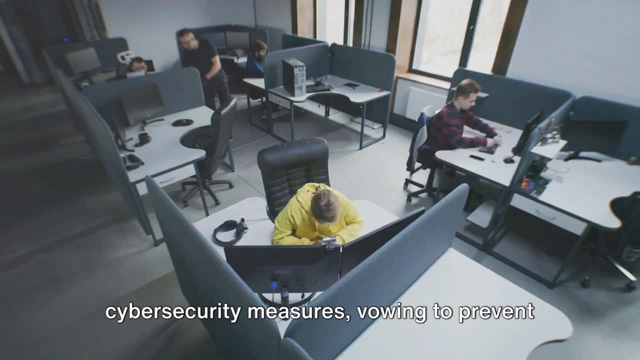 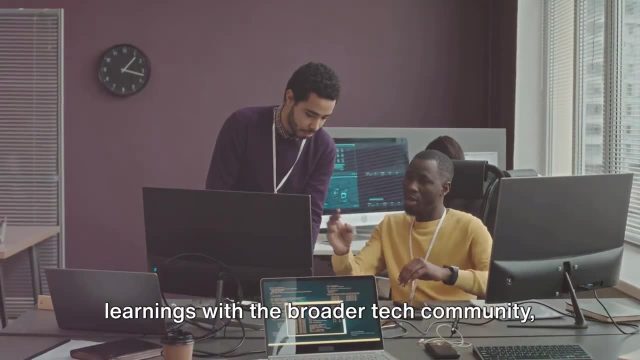 users and strengthen their cybersecurity. In the days and months that followed, Microsoft worked tirelessly to regain the trust of their users and strengthen their cybersecurity measures, vowing to prevent such a breach from occurring again. They shared their experiences and learnings with the broader tech community in a bid to raise 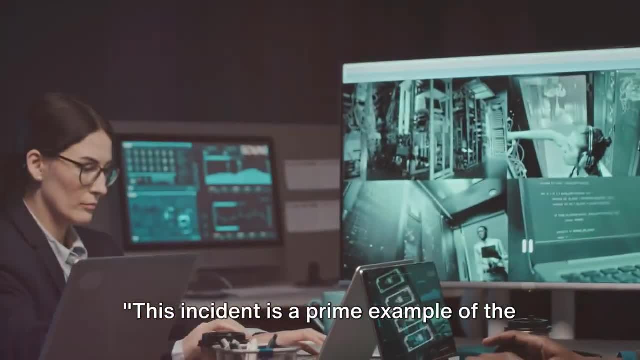 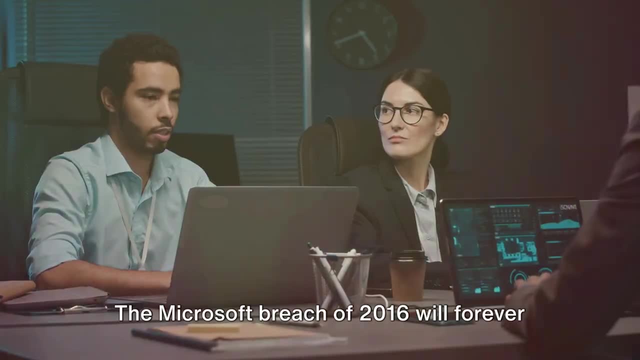 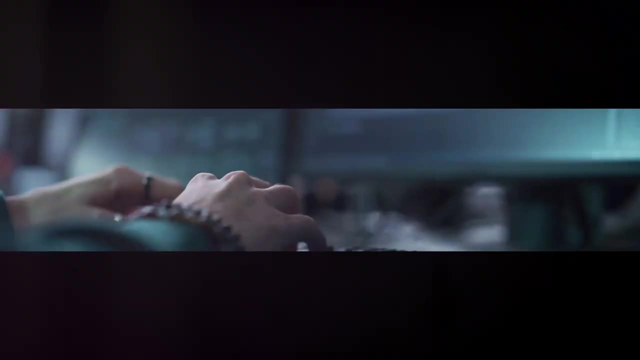 awareness and fortify the industry against similar attacks in the future. This incident is a prime example of the devastating effects of a buffer overflow attack. The Microsoft breach of 2016 will forever be etched in the annals of cybersecurity history: the digital shadows. 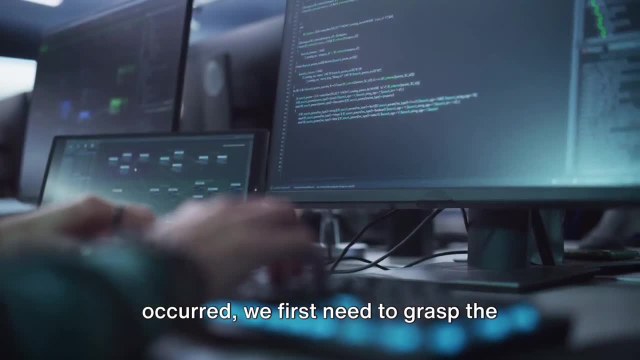 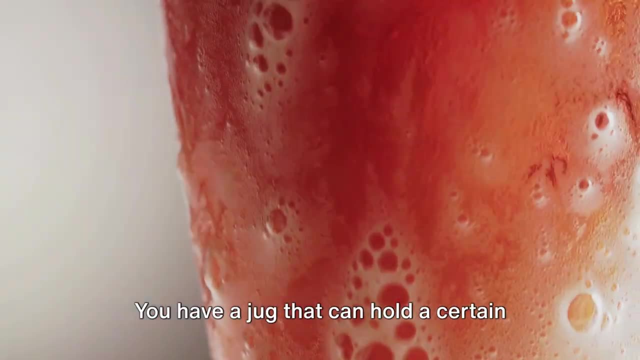 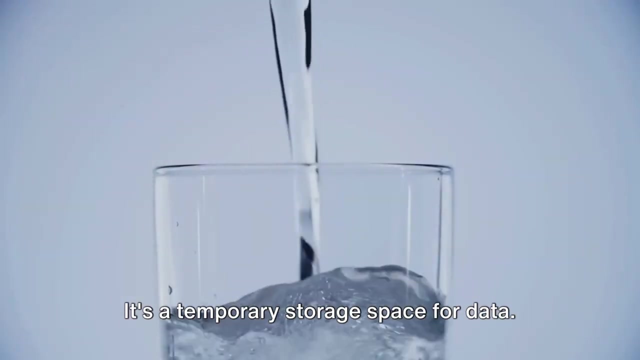 To understand how such a breach occurred, we first need to grasp the concept of a buffer overflow. Imagine you're at a party and you're pouring drinks for your friends. You have a jug that can hold a certain amount of juice. This jug is like a buffer in computing: It's a temporary storage space for data. 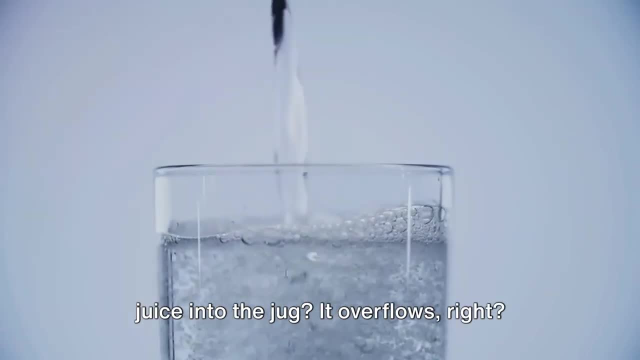 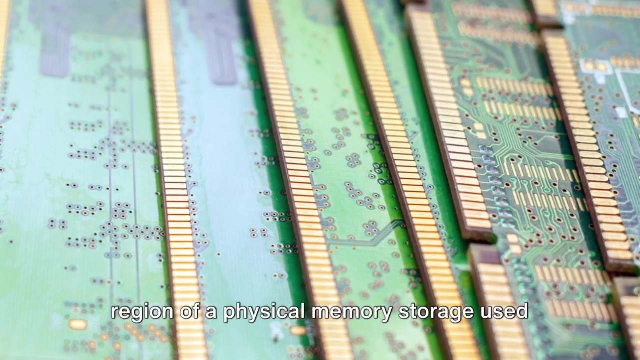 But what happens if you pour too much juice into the jug? It overflows, right, And that's exactly what happens in a buffer overflow situation In the world of computing. a buffer is a region of a physical memory storage used to temporarily hold data while 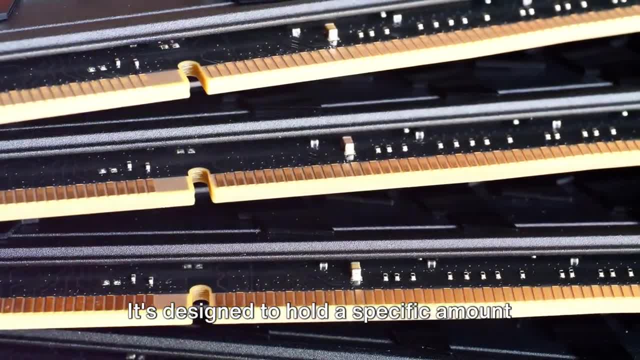 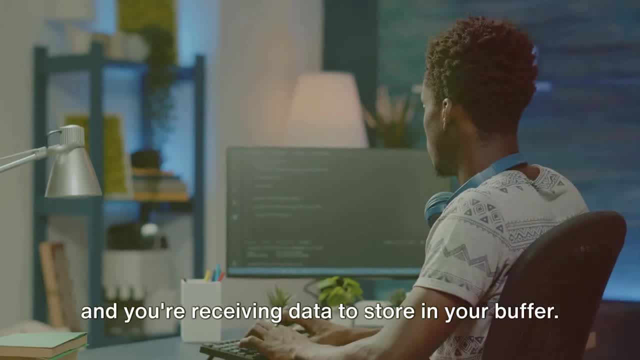 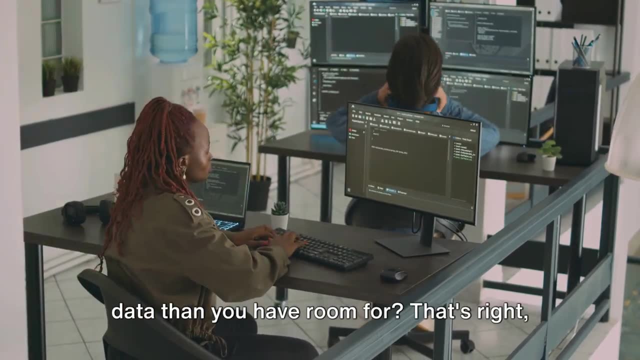 it's being moved from one place to another. It's designed to hold a specific amount of data, just like our jug of juice. Now let's imagine that you're a program and you're receiving data to store in your buffer. You're expecting a certain amount of data, but what happens if you receive more data? 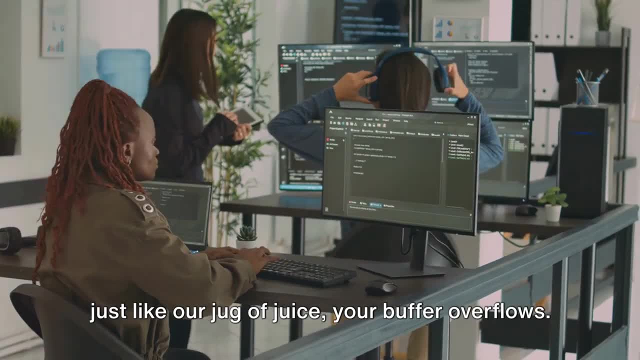 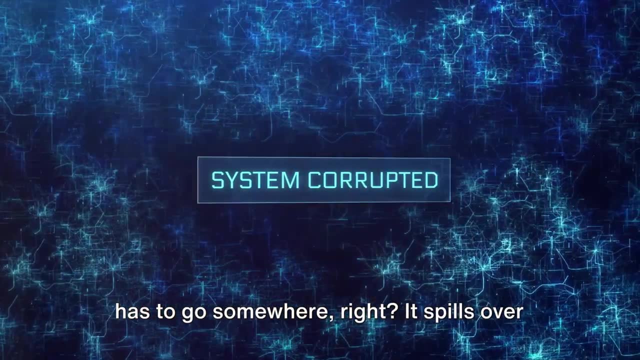 than you have room for. That's right. Just like our jug of juice, your buffer overflows. When a buffer overflows, the extra data has to go somewhere, right. It spills over into adjacent buffers, corrupting or overwriting the valid data held in them. 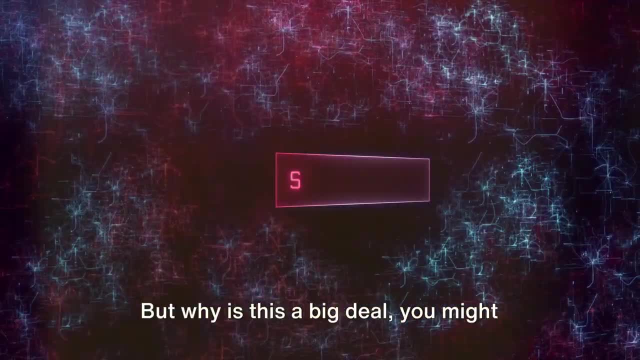 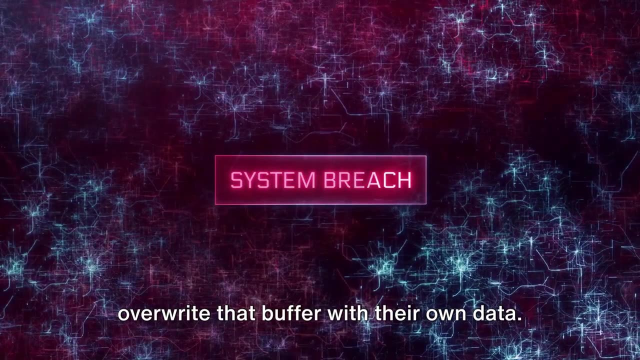 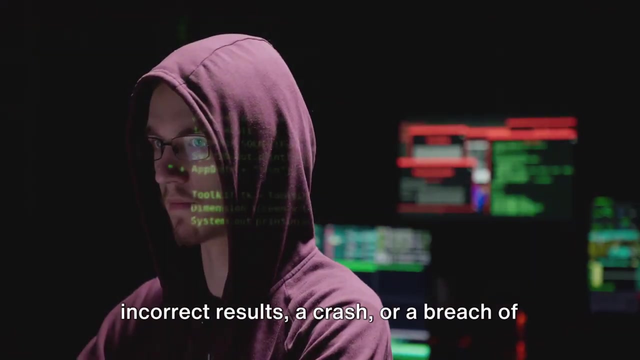 This is the essence of a buffer overflow vulnerability. But why is this a big deal, you might ask? Well, if a hacker can intentionally cause a buffer overflow, they can overwrite that buffer with their own data. This can lead to erratic program behavior, including memory access errors, incorrect results, a crash or a breach of security. 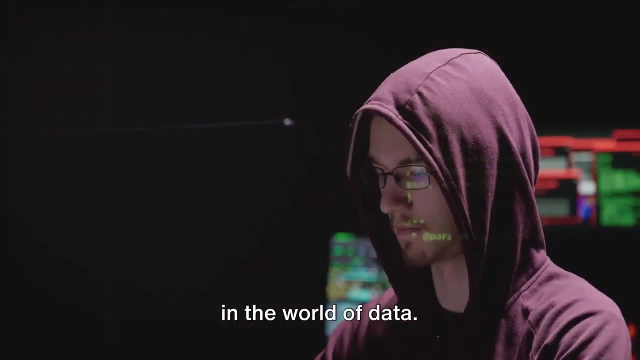 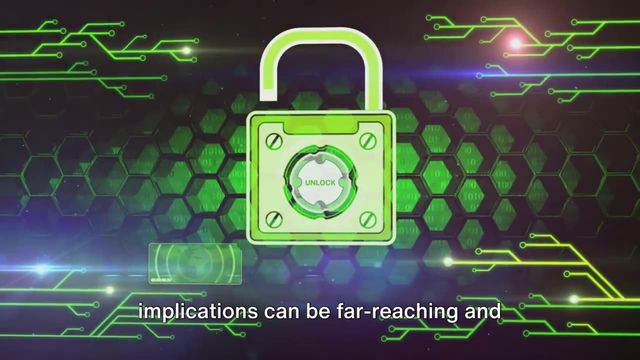 In essence, it's like a dam bursting, but in the world of data, And that's a buffer overflow. in a nutshell, It's a simple concept, but its implications can be far reaching and potentially devastating in the wrong hands. In essence, a buffer overflow is like a dam bursting. 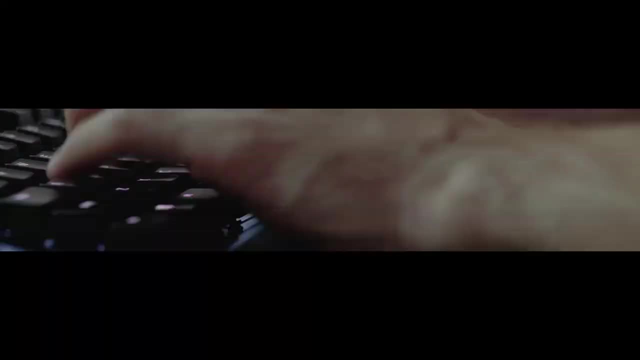 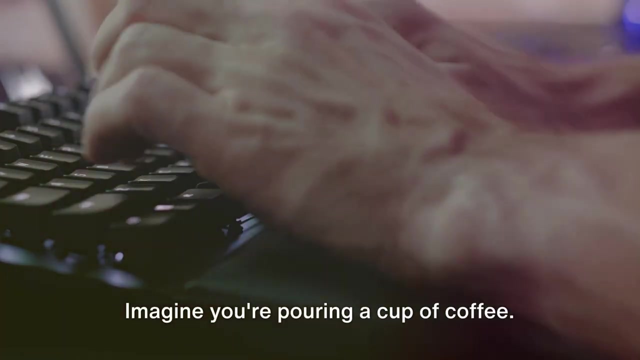 but in the world of data. Now that we have a basic understanding, let's delve deeper into how a buffer overflow actually works. Imagine you're pouring a cup of coffee. If you pour too much, it overflows right away. But what happens if you pour too much? 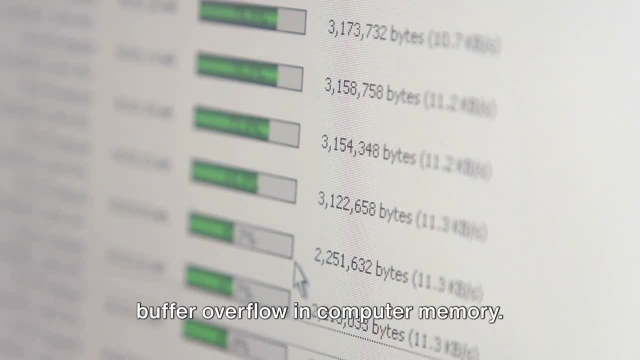 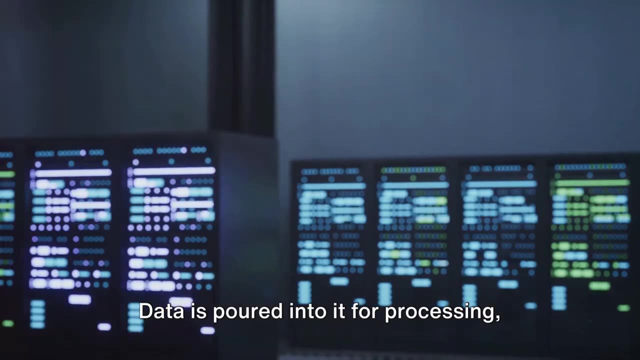 The same principle applies to buffer overflow in computer memory. In the world of computing, a buffer is a temporary storage space, sort of like a coffee cup. Data is poured into it for processing. but what happens when there's too much data? Well, just like the coffee cup, the buffer overflows. 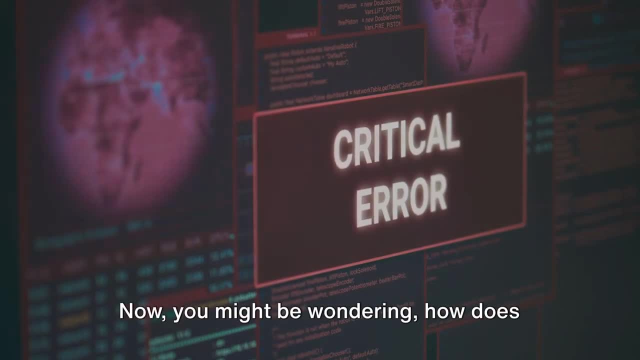 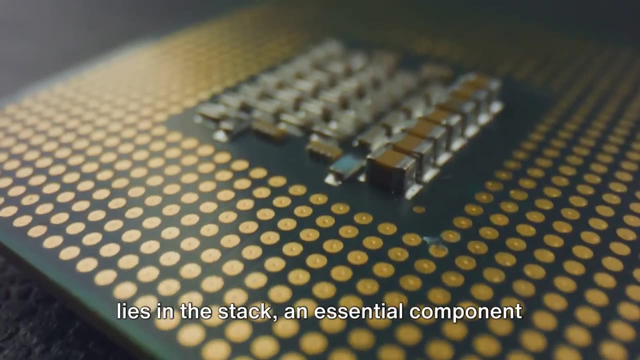 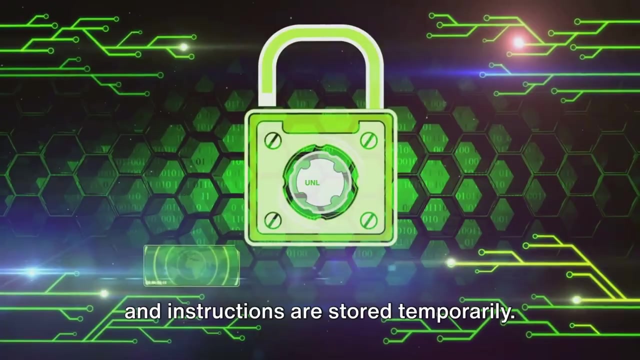 This overflow can lead to data corruption or even a system crash. Now you might be wondering how does this overflow actually occur? The answer lies in the stack, an essential component of a computer's memory. A stack is a region of memory where data and instructions are stored temporarily. It grows. 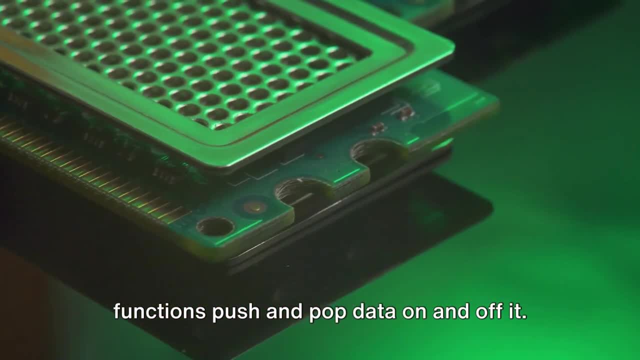 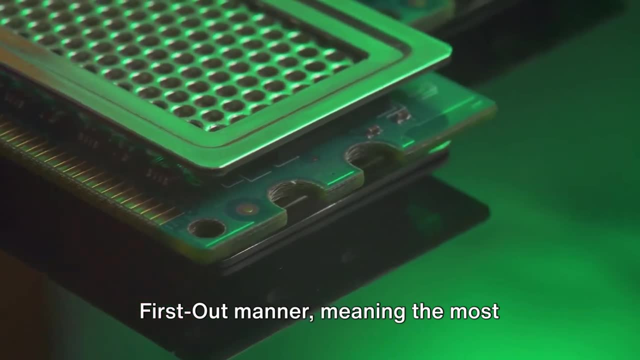 and shrinks automatically as functions push and pop data on and off it. Here's where things get interesting. The stack stores data in a last-in, first-out manner, meaning the most recently stored data will be the first to be retrieved. However, if a function attempts to push more data onto the 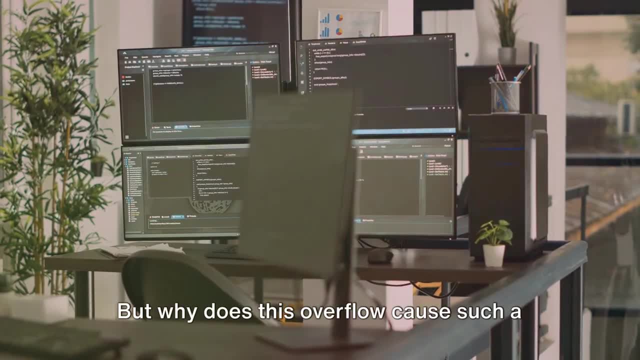 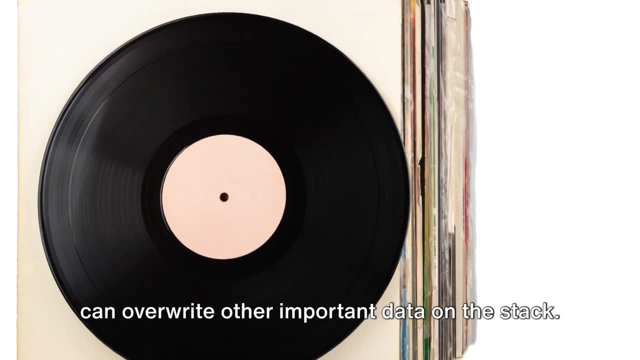 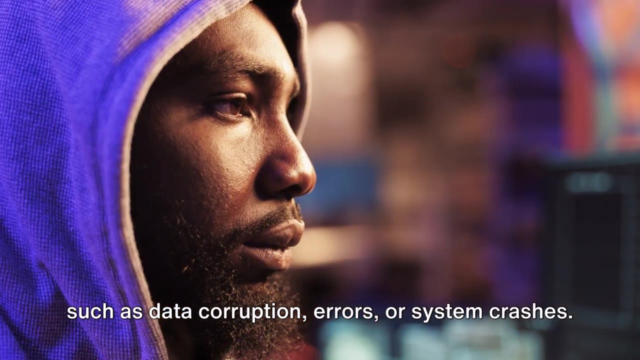 stack than it can handle. we experience a buffer overflow. But why does this overflow cause such a problem? Well, the overflowing data can overwrite other important data on the stack. This can lead to unpredictable behavior such as data corruption, errors or system crashes. Worse yet, if an 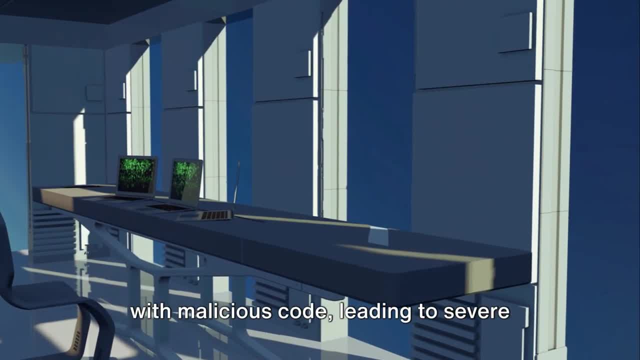 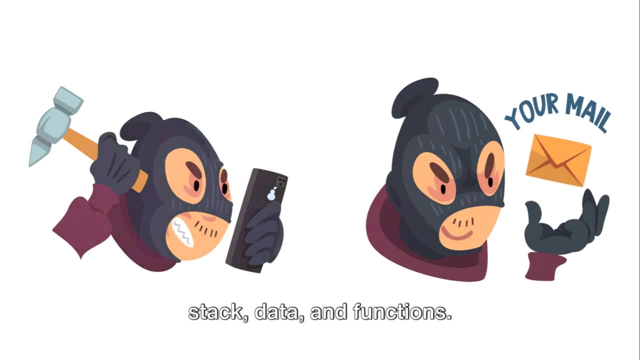 attacker can control the overflow, they can overwrite the stack with malicious code, leading to severe security breaches. So the mechanics of buffer overflow involve a delicate interplay between the stack data and functions. There's a careful balance to be maintained here, A balance that, when tipped, 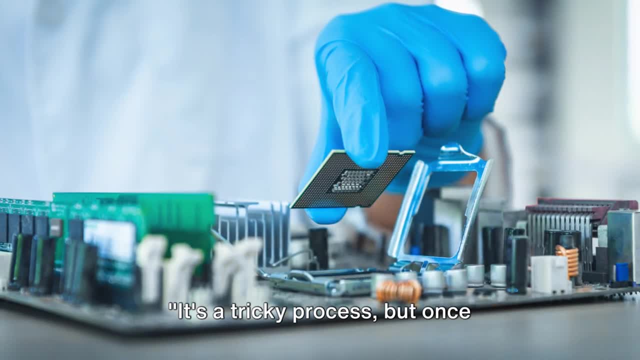 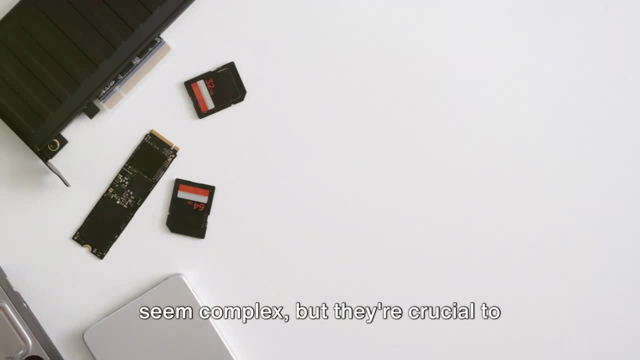 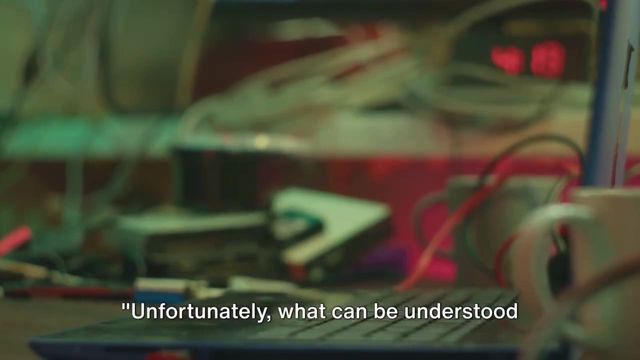 can lead to significance issues. It's a tricky process but, once understood, it paints a clear picture of how data can be compromised. The mechanics of buffer overflow might seem complex, but they're crucial to understanding how systems can be made vulnerable and how we can better protect them. Unfortunately, what can be? 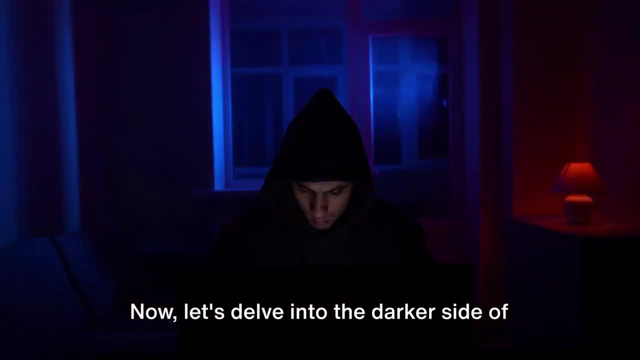 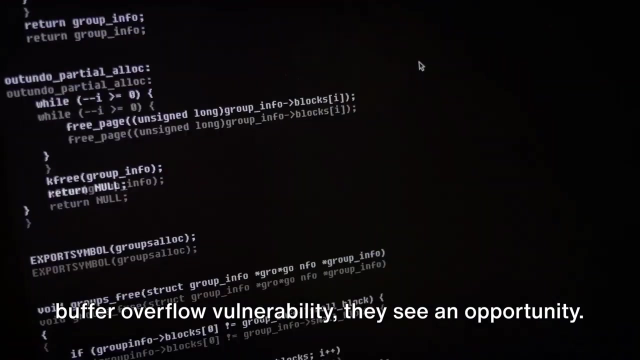 understood, can also be exploited. Now let's delve into the darker side of buffer overflow. It's not just a technical glitch or a programming error. it becomes a lethal weapon in the hands of a skilled hacker. You see, when a hacker identifies a buffer overflow vulnerability, they see an opportunity, An 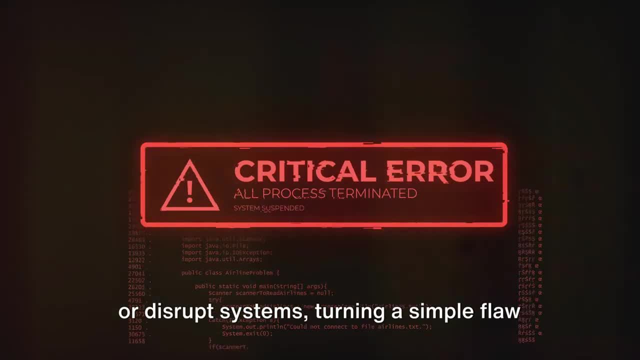 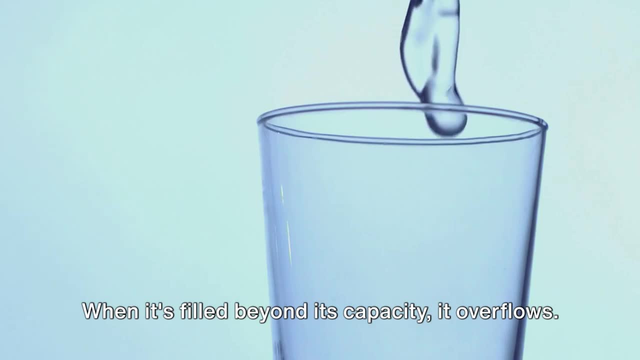 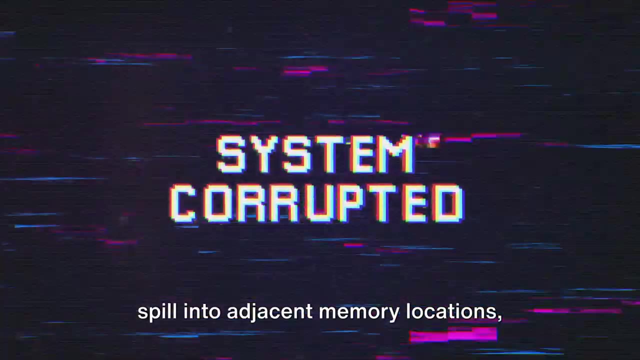 opportunity to execute malicious code or disrupt systems, turning a simple flaw into a potent tool for chaos. Imagine a buffer as a glass of water: When it's filled beyond its capacity, it overflows In a computer system. this overflow can spill into adjacent memory locations, corrupting or even overwriting the 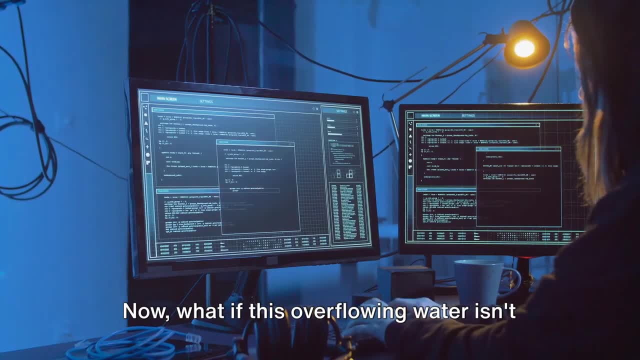 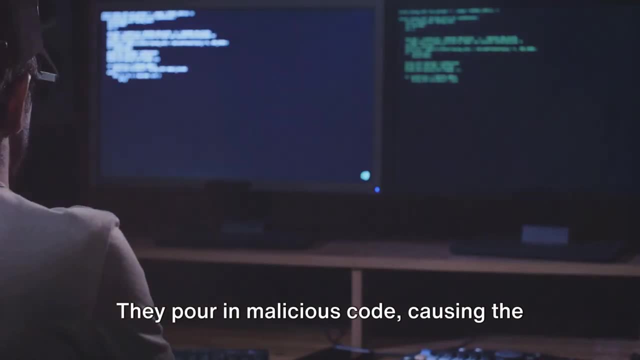 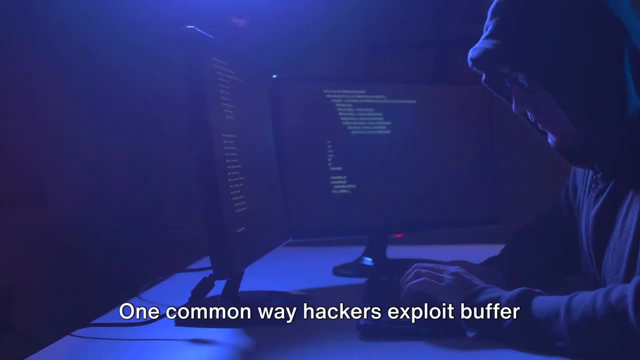 data stored there. now, what if this overflowing water isn't just water but a specially crafted poison? that's what a hacker does: they pour in malicious code, causing the system to behave unpredictably or, even worse, in a manner that the hacker desires. one common way hackers exploit: 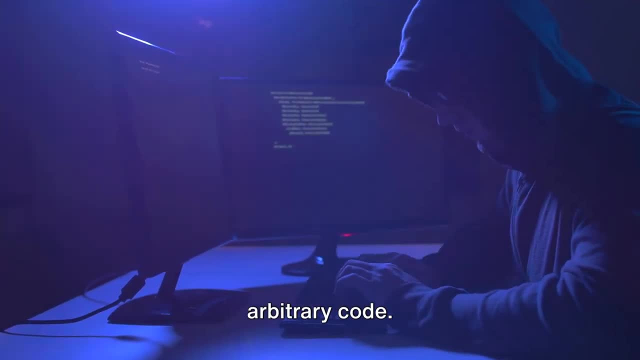 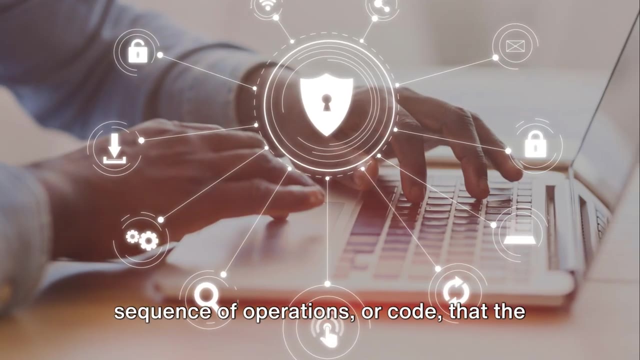 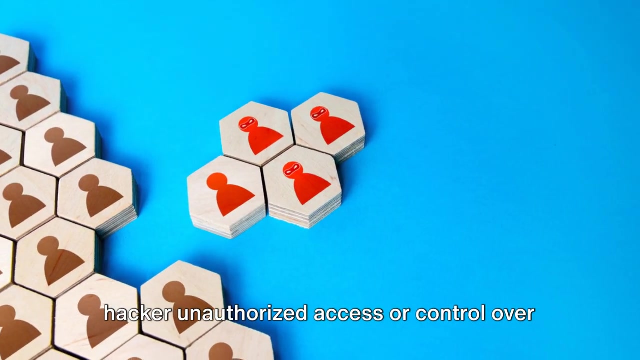 buffer overflow is through the execution of arbitrary code. the hacker carefully crafts input data which, when overflowed, contains a specific sequence of operations or code that the system will execute. this could include actions that grant the hacker unauthorized access or control over the system. another method is the denial of service attack, or dos. 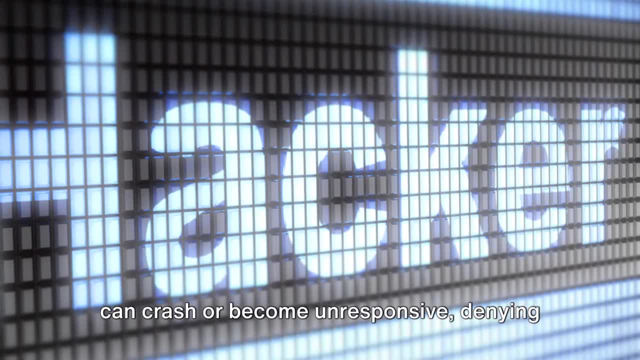 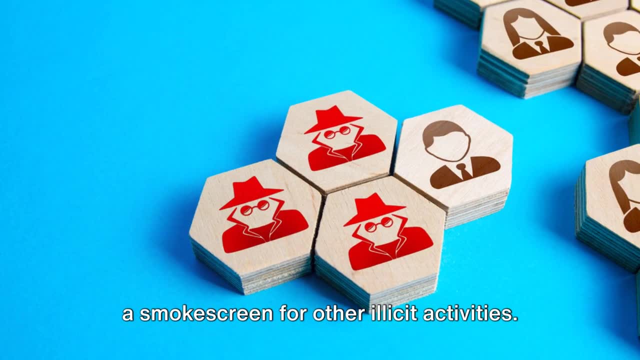 by causing a buffer overflow. the system can crash or become unresponsive, denying service to legitimate users. this is often done to distract or create a smoke screen for other illicit attacks. the system can crash or become unresponsive, denying service to legitimate users. this is often done to distract or create a smoke screen for other illicit attacks. 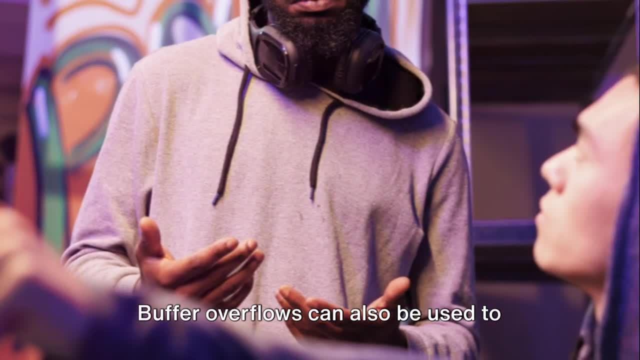 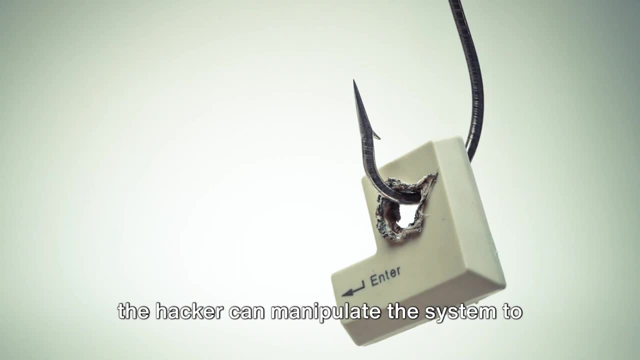 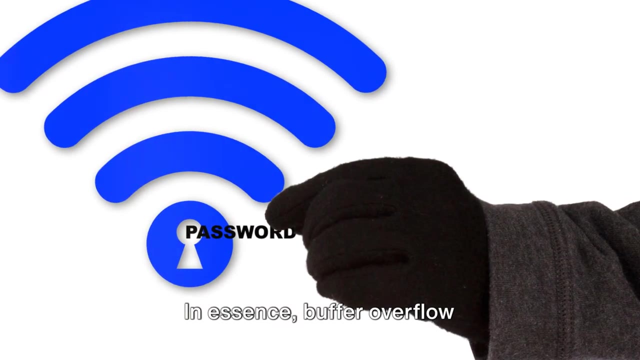 it activities. buffer overflows can also be used to alter the program's flow of execution. by overwriting certain memory locations, the hacker can manipulate the system to skip security checks or execute functions it wouldn't normally perform. in essence, buffer overflow vulnerabilities provide hackers a foothold, a backdoor into systems, allowing them to infiltrate. 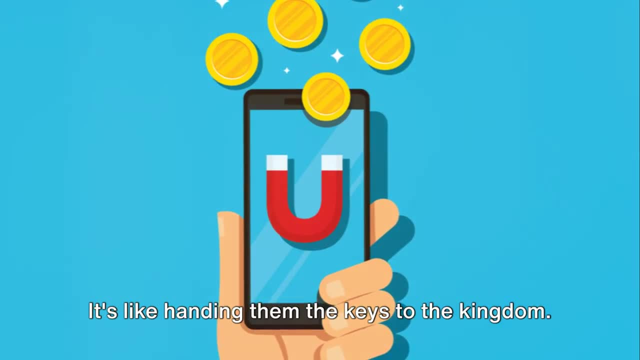 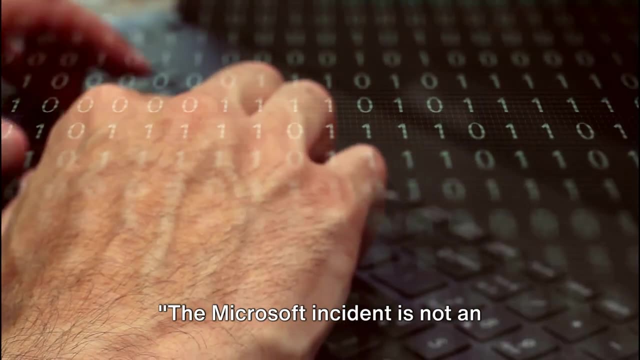 disrupt and control. it's like handing them the keys to the kingdom buffer overflow. it's like handing them the keys to the kingdom buffer overflow. in the hands of a hacker becomes a potent tool for chaos. the microsoft incident is not an isolated one. let's delve into the murky waters. 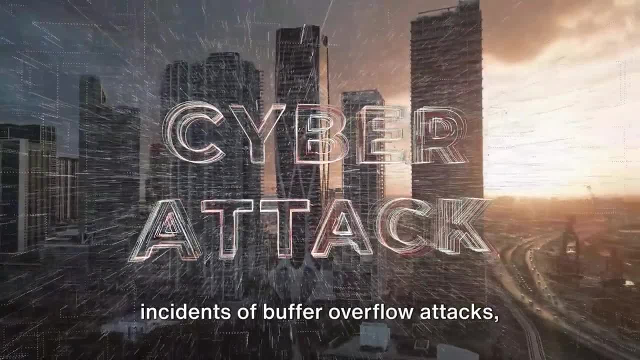 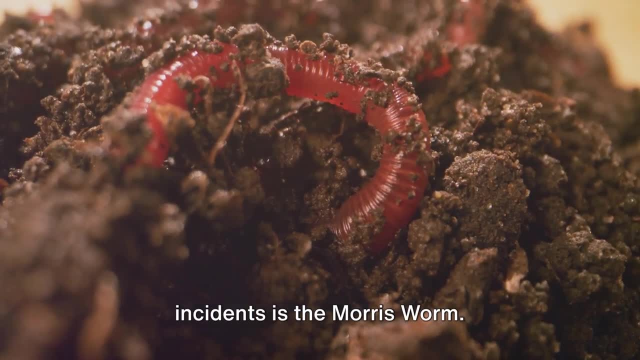 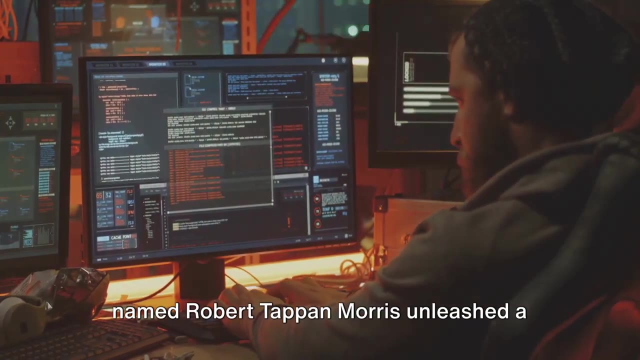 of cyberspace to recount other notorious incidents of buffer overflow attacks which have left indelible marks in the annals of cyber security. perhaps one of the most infamous incidents is the morris worm. in 1988, a 23 year old graduate student named robert tappan morris unleashed a worm that was 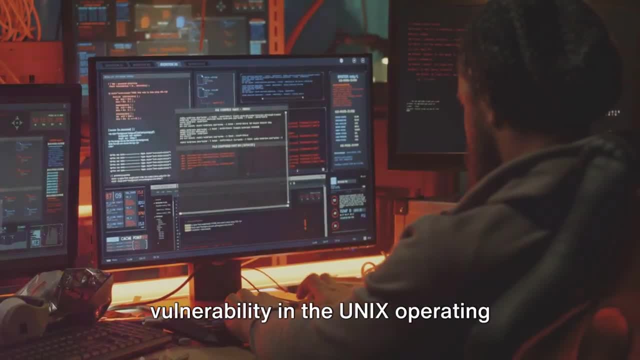 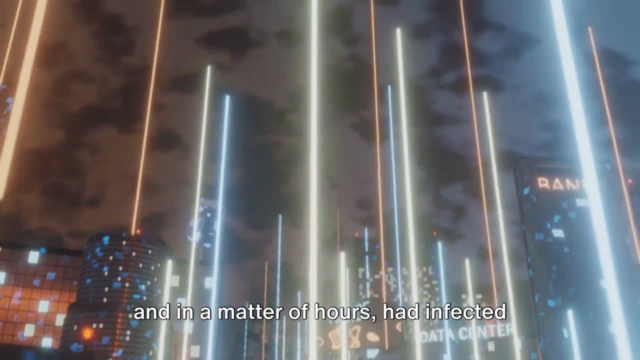 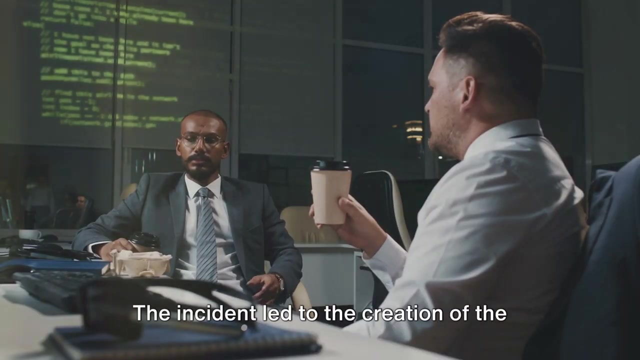 that exploited a buffer overflow vulnerability in the unix operating system's finger demon. the worm replicated at an alarming rate and in a matter of hours had infected around 6 000 machines, which was approximately 10 percent of the entire internet. back then, the incident led to the 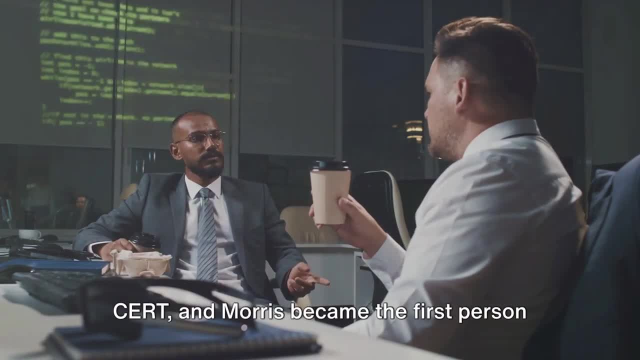 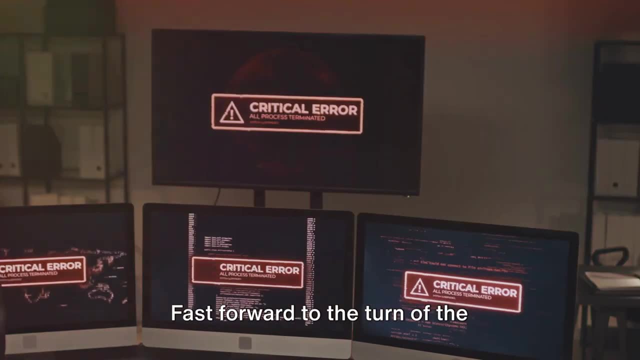 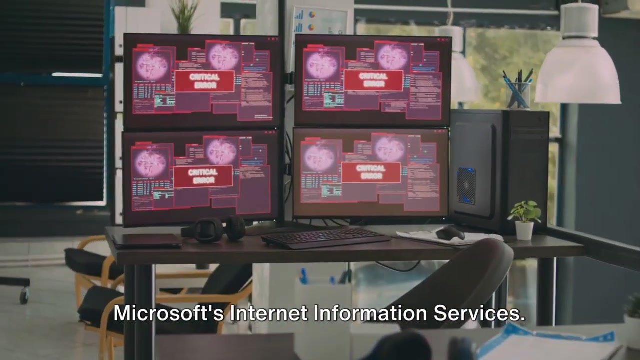 creation of the first computer emergency response team, or cert, and morris became the first person convicted under the computer fraud and abuse act. fast forward to the turn of the millennium, the code red worm exploited a buffer overflow vulnerability in microsoft's internet information services. in less than a week, the worm infected nearly 400 000 servers. 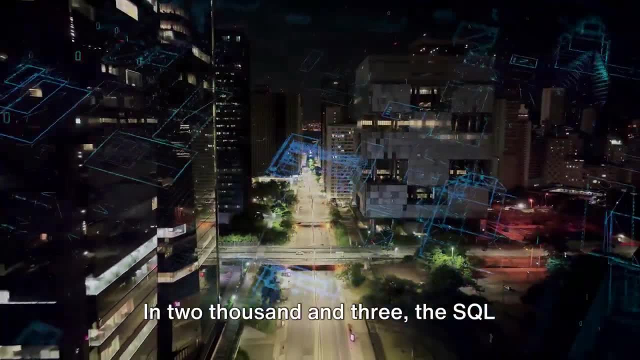 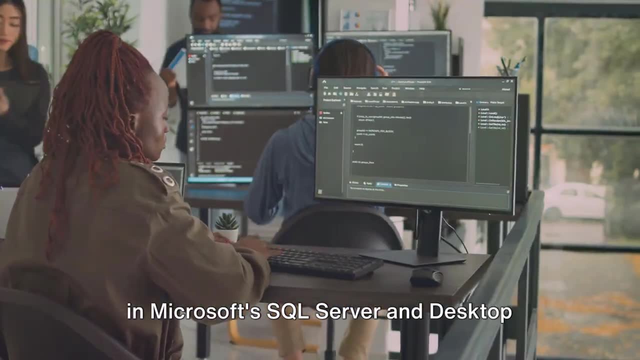 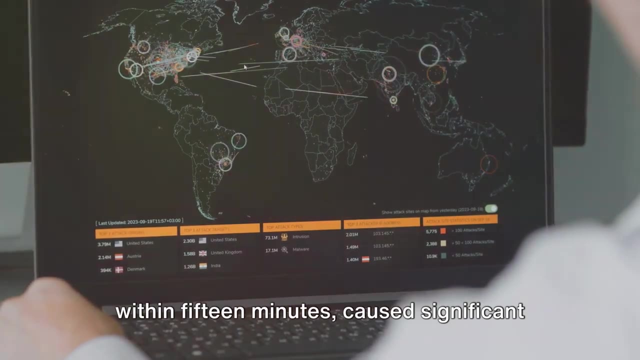 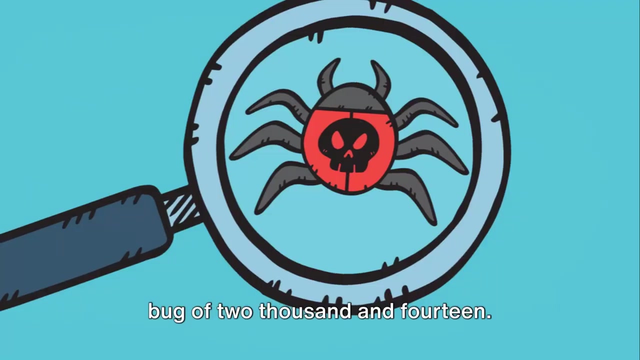 defacing websites and launching denial of service attacks. in 2003, the sql slammer worm exploited a buffer overflow in microsoft's sql server and desktop engine database products. it doubled in size every few seconds and within 15 minutes caused significant internet slowdown globally. then, of course, there's the heartbleed bug of 2014.. it exploited a buffer 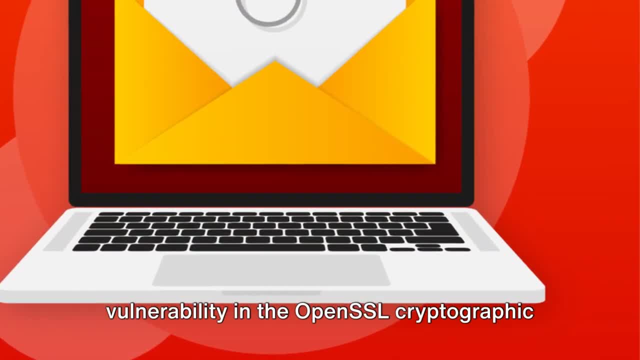 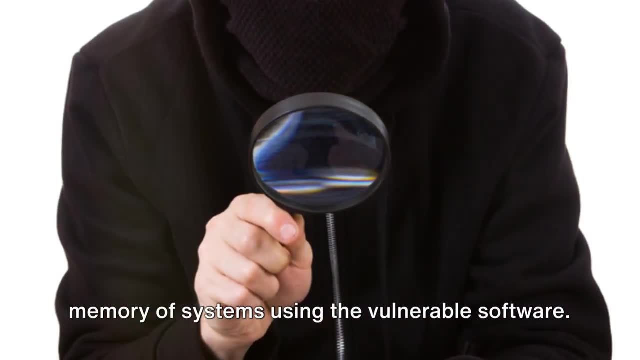 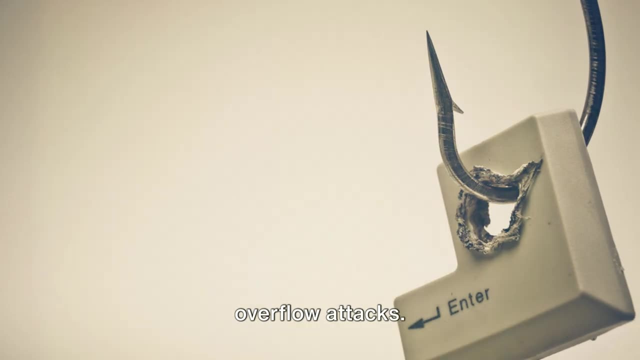 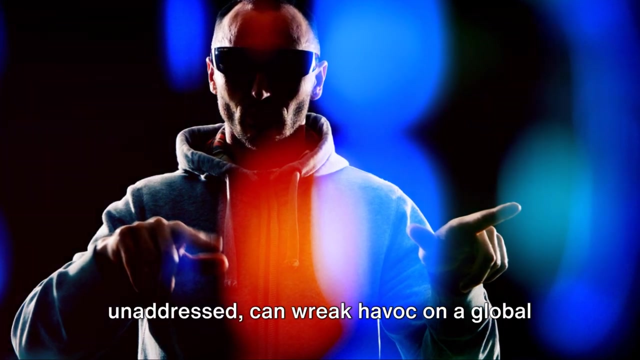 overflow vulnerability in the open ssl cryptographic software library, potentially allowing attackers to read sensitive data from the memory of systems using the vulnerable software. these incidents underscore the widespread and destructive potential of buffer overflow attacks. they serve as stark reminders that buffer overflow vulnerabilities, if used left unaddressed, can wreak havoc on a global scale, compromising systems, stealing sensitive. 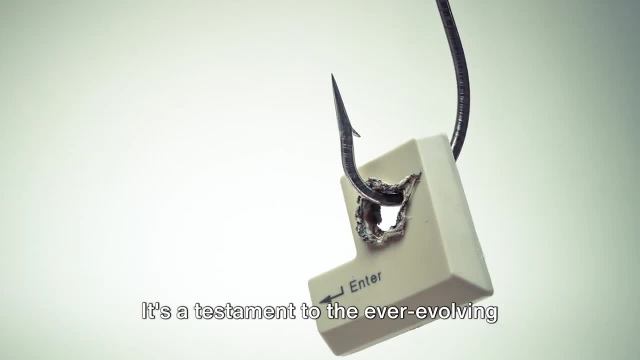 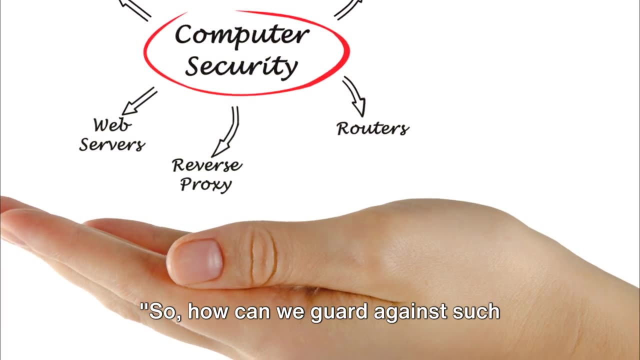 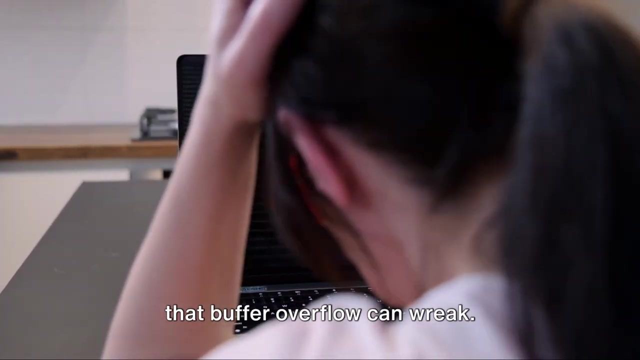 data and even bringing the internet to a standstill. it's a testament to the ever-evolving nature of cyber threats and the constant need for diligent security measures. so how can we guard against such attacks? it's a question that naturally springs to mind after seeing the havoc that buffer overflow. 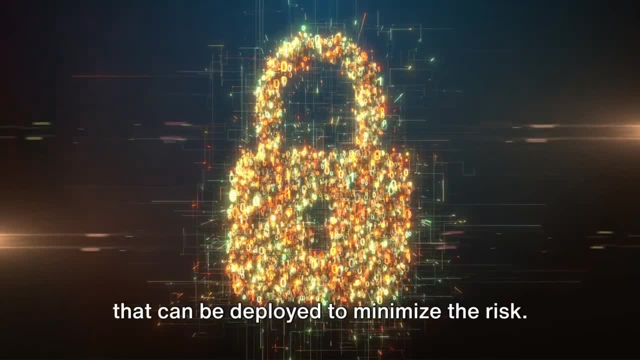 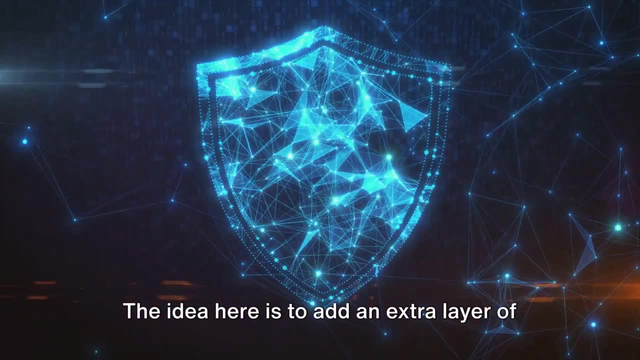 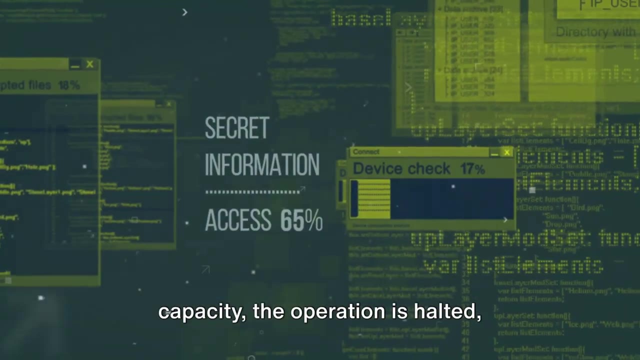 can wreak. thankfully, there are several strategies that can be deployed to minimize the risk. first up is bound checking. the idea here is to add an extra layer of security that verifies the amount of data being written into a buffer. if the data exceeds the buffer's capacity, the 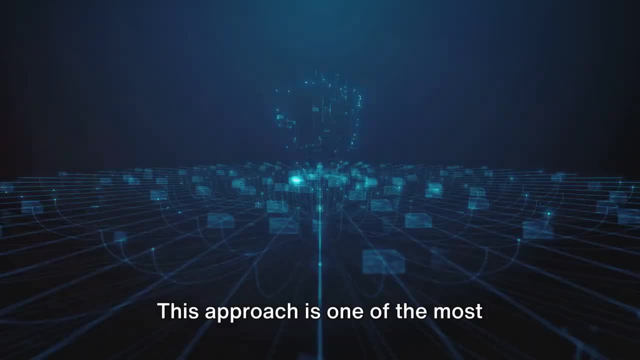 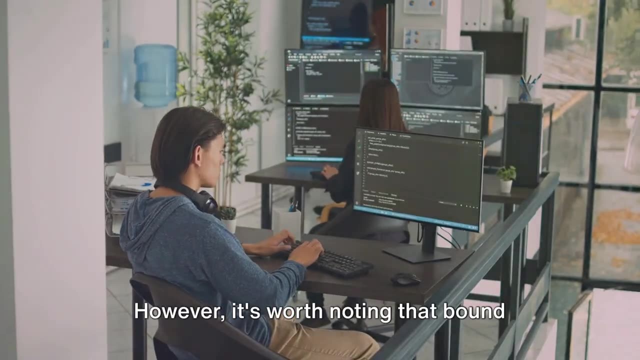 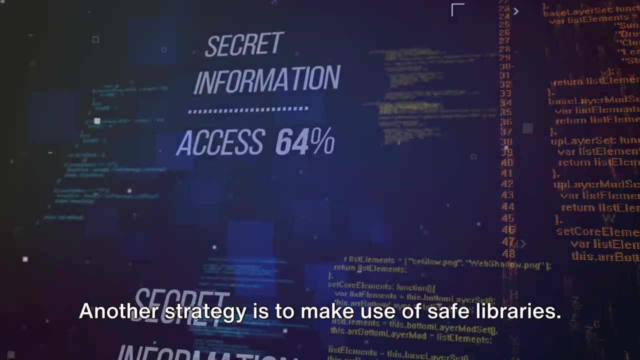 operation is halted, preventing a buffer overflow. this approach is one of the most effective ways to stop buffer overflow attacks in their tracks. however, it's worth noting that bound checking does come with a slight performance cost due to the extra checks. it necessitates another change in the ability of the data storage to ensure that the data is stored properly. 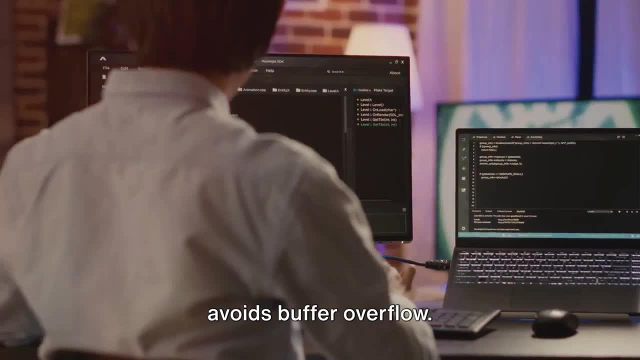 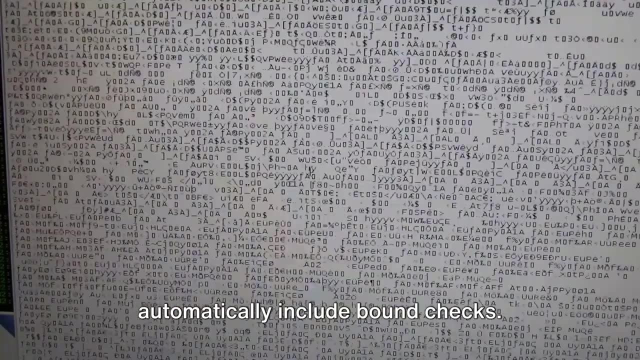 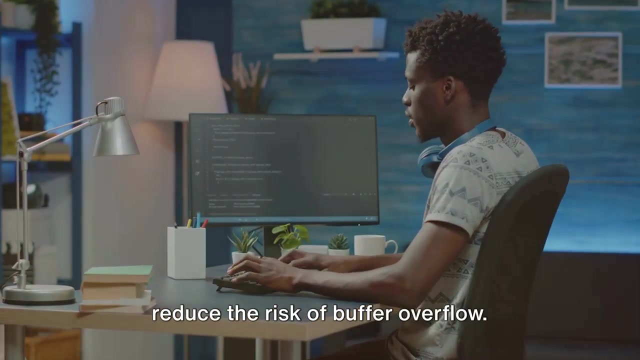 the third strategy is to make use of safe libraries. these libraries have been specifically designed to handle data in a way that avoids buffer overflow. they replace standard susceptible functions with safer alternatives that automatically include bound checks. by substantiating your code with these safer functions, you can drastically reduce the risk of buffer overflow. additionally, randomizing: 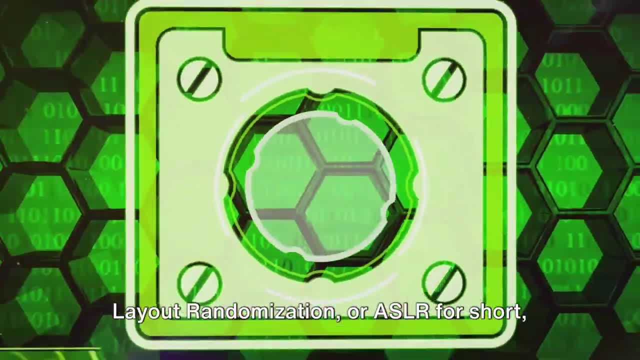 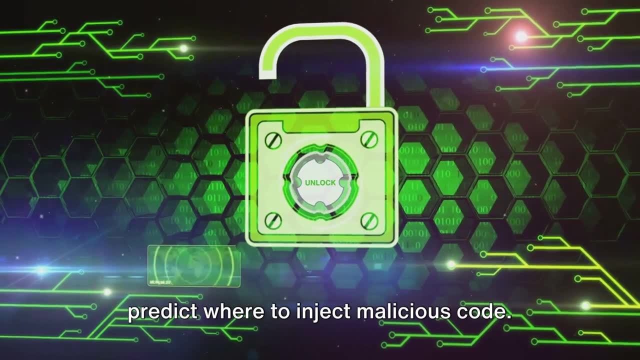 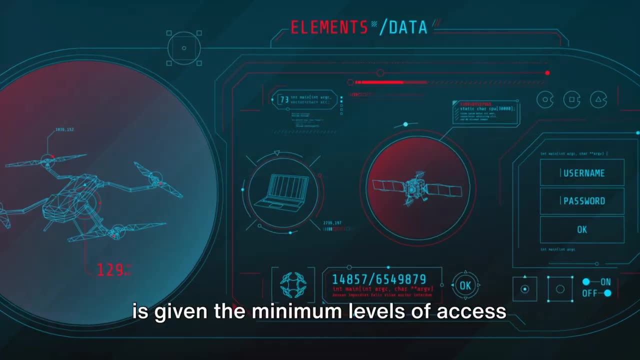 useful tactic. This method, known as Address Space Layout Randomization, or ASLR for short, makes it much harder for an attacker to predict where to inject malicious code. Finally, there's the principle of least privilege. This is a security concept where a user is given 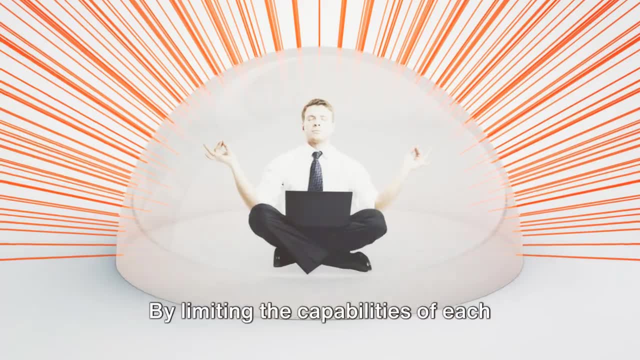 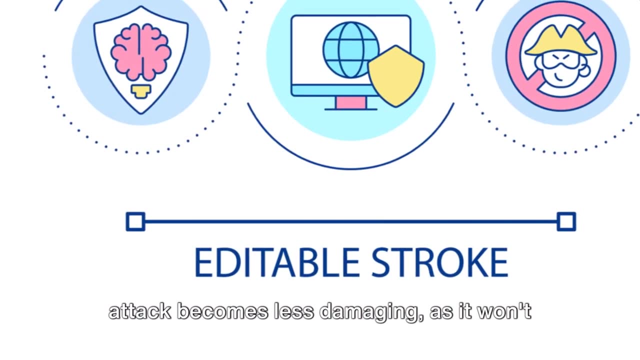 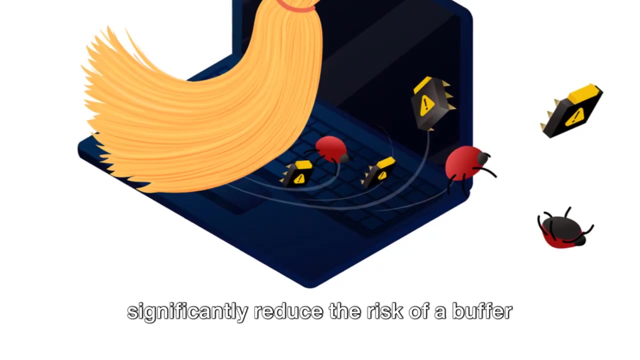 the minimum levels of access necessary to perform their tasks. By limiting the capabilities of each program, any potential buffer overflow attack becomes less damaging, as it won't have the permissions to alter critical areas of the system. These measures, while not foolproof, can significantly reduce the risk of a buffer overflow attack. It's important to remember 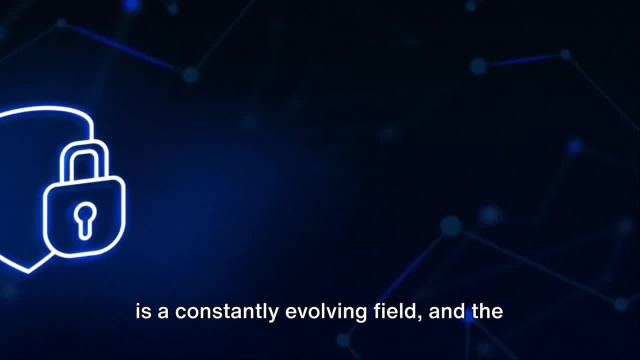 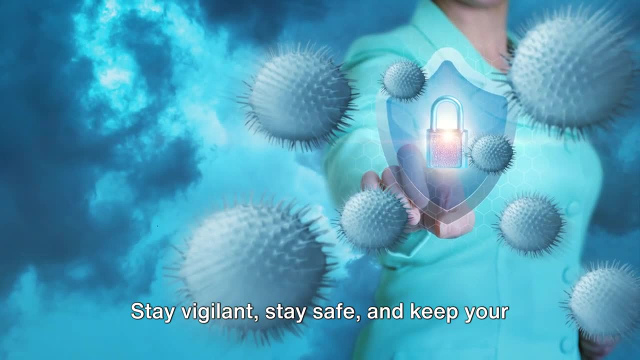 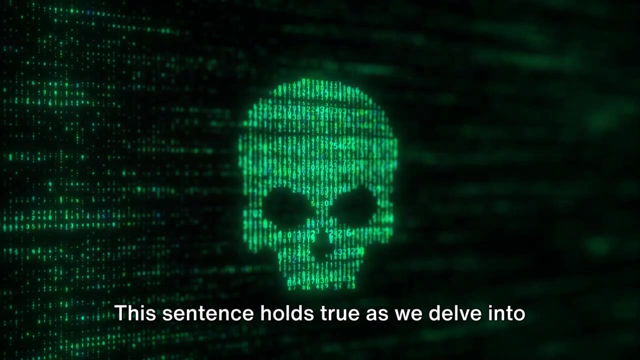 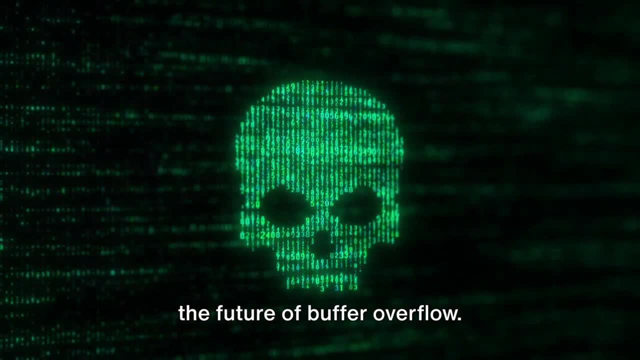 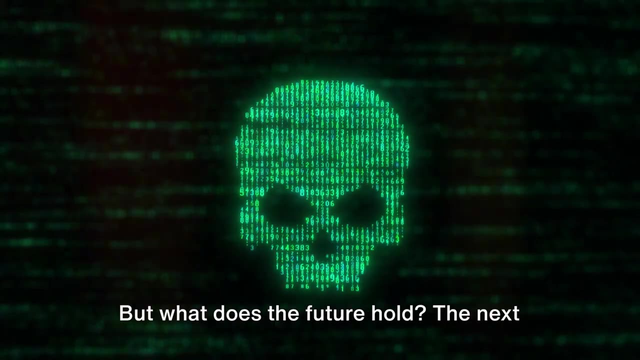 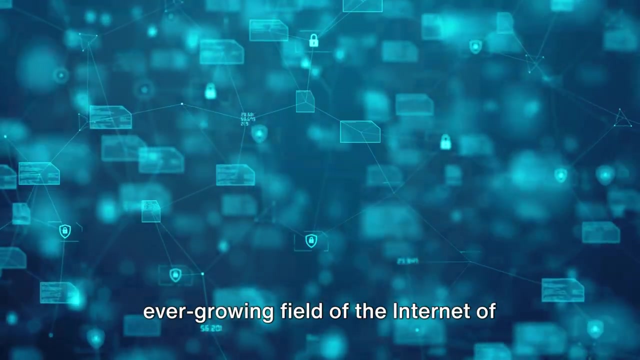 This sentence holds true as we delve into the future of buffer overflow. Buffer overflow attacks have been around for decades and they've adapted to the changes in technology, But what does the future hold? The next frontier for these attacks could be the ever-growing field of the Internet of Things. 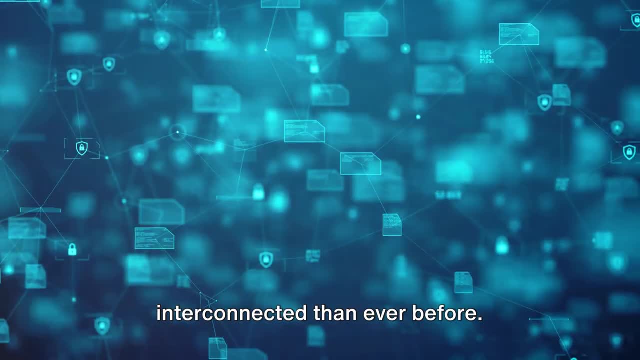 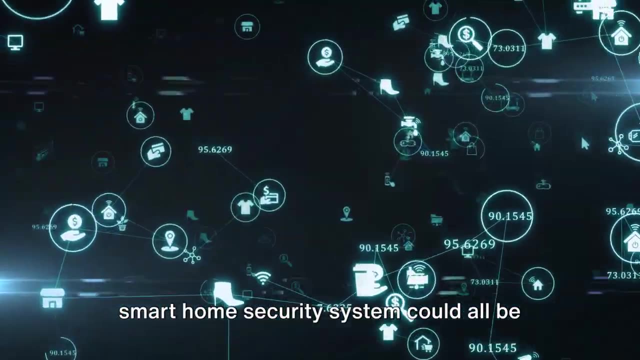 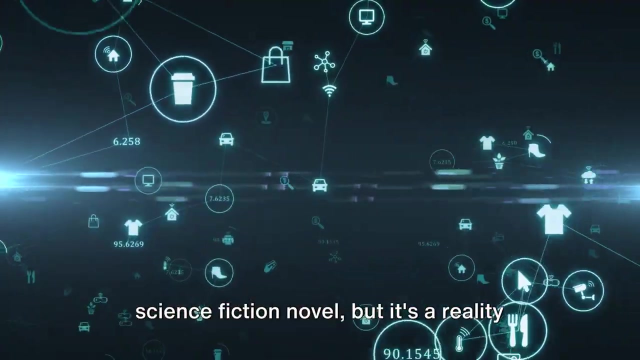 or IoT, where devices are more interconnected than ever before. Imagine a world where your smart fridge, your wearable fitness tracker or your smart home security system could all be potential targets for buffer overflow attacks. Yes, it sounds like something out of a science fiction novel. 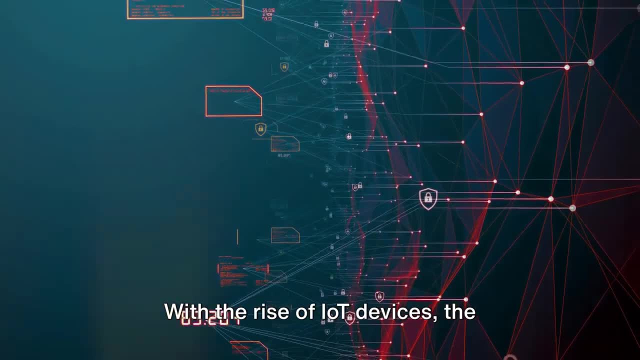 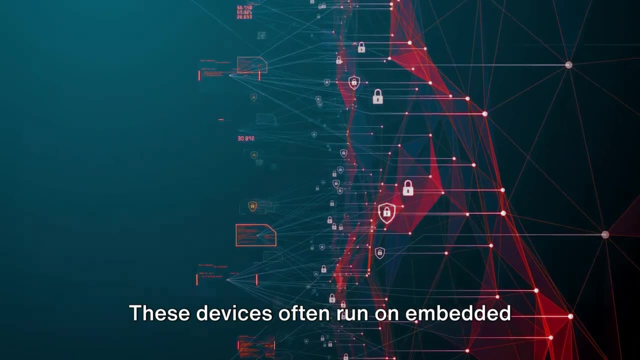 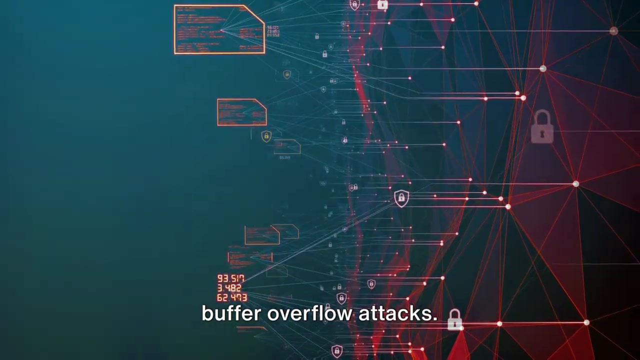 but it's a reality we need to prepare for. With the rise of IoT devices, the potential attack surface for hackers expands exponentially. These devices often run on embedded systems with limited memory and computing power, making them prime targets for buffer overflow attacks. The fact that many of these devices lack proper security measures only adds to the problem. Moreover, the increased use of artificial intelligence and machine learning in cyber defenses presents a double-edged sword. While these technologies can help detect and prevent attacks, they can also be exploited by hackers. Advanced buffer overflow attacks could potentially manipulate machine learning models, leading to false positives or worse. 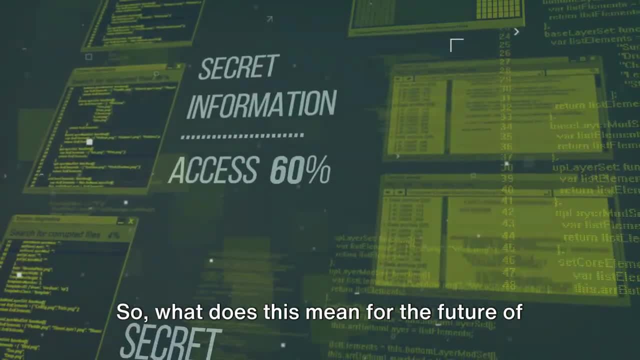 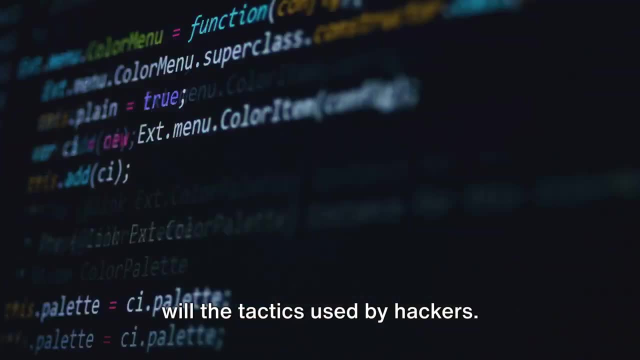 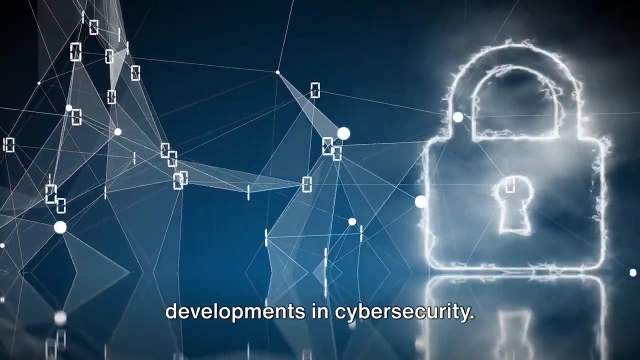 going undetected. So what does this mean for the future of buffer overflow? It means that as technology continues to evolve, so too will the tactics used by hackers. It means that we need to stay vigilant, constantly updating our defenses and staying informed about the latest developments in 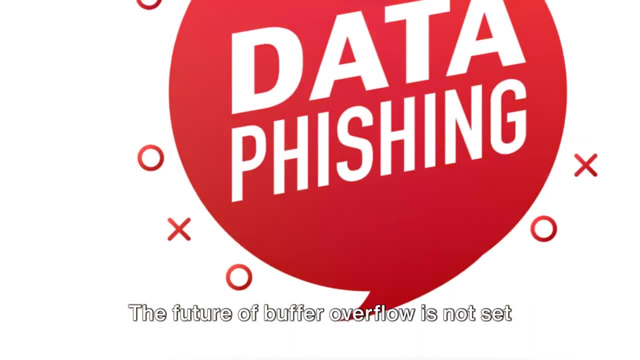 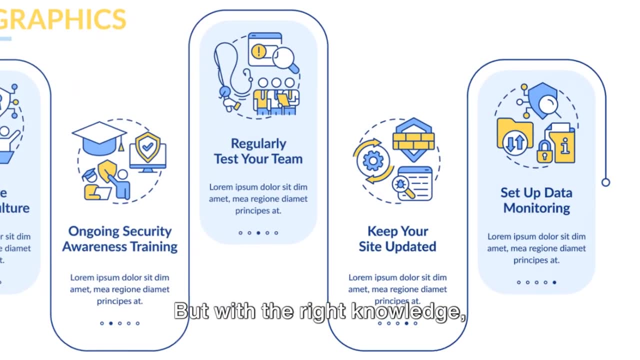 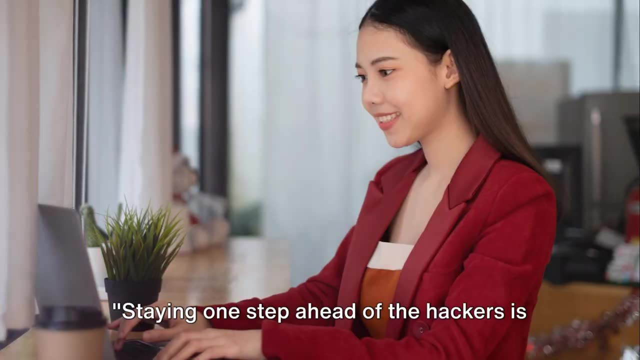 cybersecurity. The future of buffer overflow is not set in stone. It's a dynamic, ever-changing landscape that will continue to challenge us, But with the right knowledge, preparation and tools, we can mitigate the risks and stay one step ahead. Staying one step ahead of the hackers is a 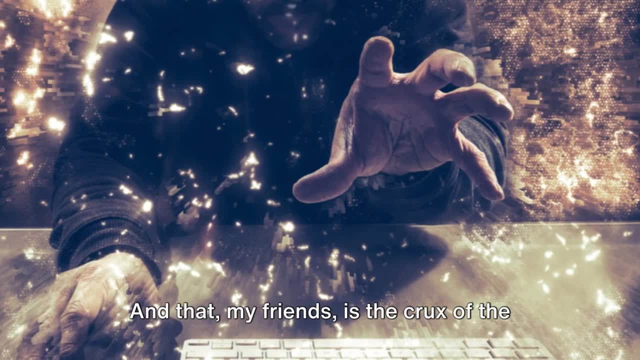 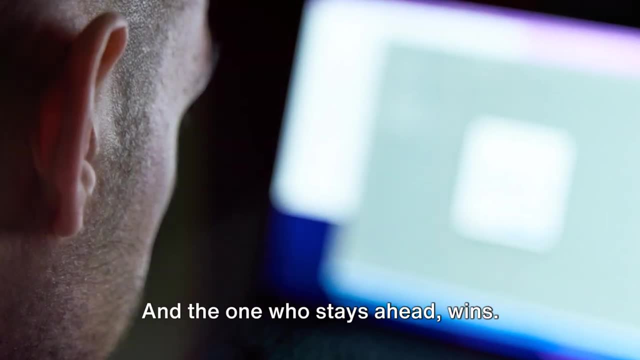 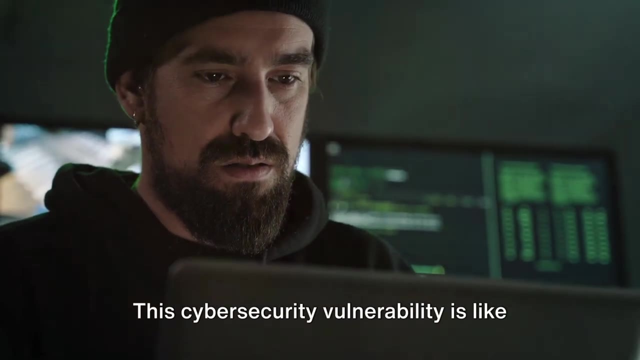 constant challenge in the world of cybersecurity And that, my friends, is the crux of the matter. The future of buffer overflow is a continuous game of cat and mouse, And the one who stays ahead wins. Before we wrap up, let's summarize what we've learned about buffer overflow. 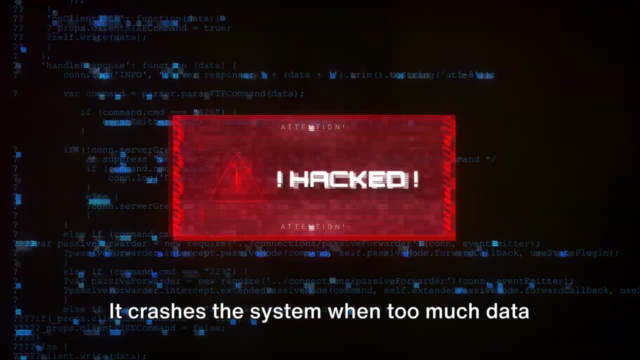 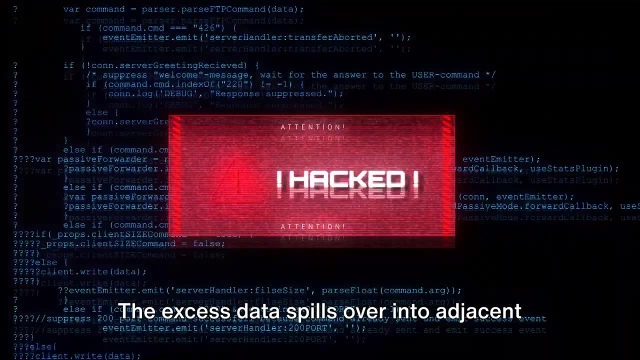 This cybersecurity vulnerability is like an uninvited guest at a party: It crashes the system. when too much data is fed into a buffer, a temporary data storage area, The excess data spills over into adjacent buffer areas. This is a constant challenge in the world of cybersecurity. 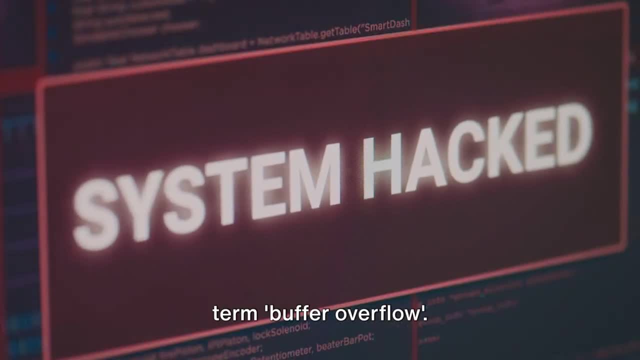 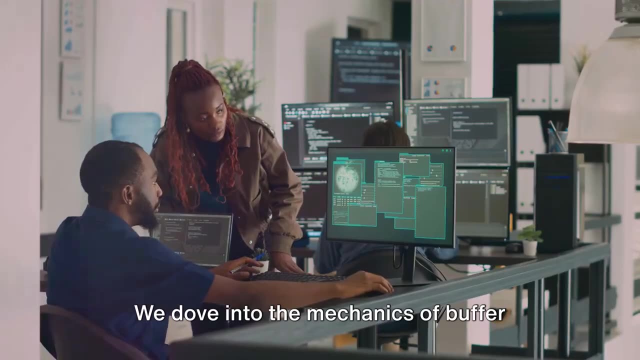 We need to continue to stand up톛k in order to offenat 여기서 If we can get the most知識. It's a sneaky technique often used by hackers to exploit systems and gain unauthorized access. We dove into the mechanics of buffer overflow. 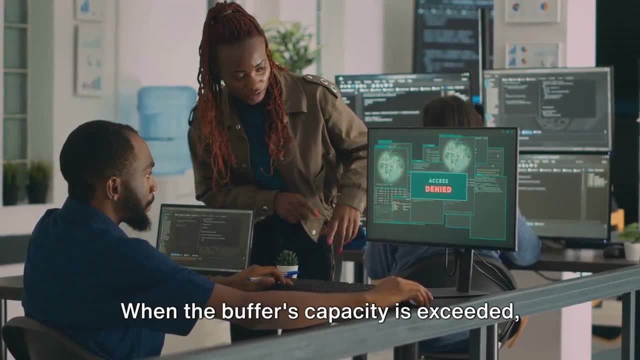 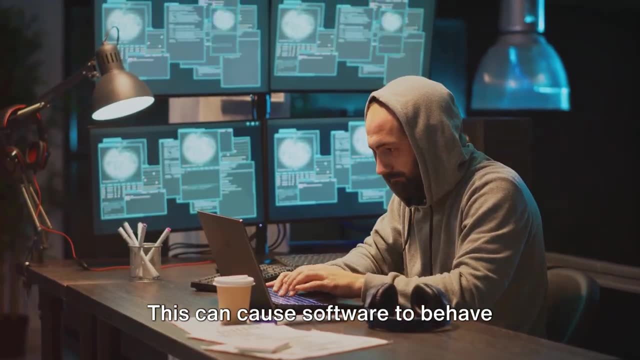 As if all replaced the most превYU OPEN UP. Now it's really quite fascinating. When the buffer's capacity is exceeded, the surplus data overflows into other buffers, sometimes overwriting important data. This can cause software to behave unpredictably, potentially leading to system crashes. 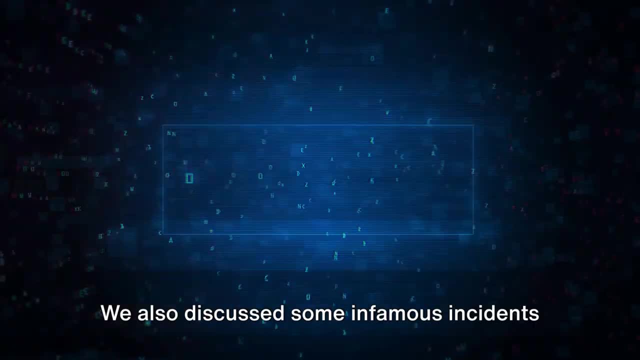 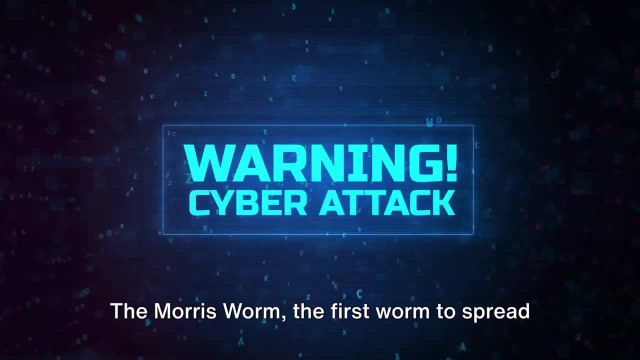 data curbs and they could turn speed on any one of the two frequent success stories in cybersecurity. Thomson v: What can a corruption and security breaches? we also discussed some infamous incidents of buffer overflow, which served as wake-up calls for the cyber security world. the morris worm: the first worm to spread. 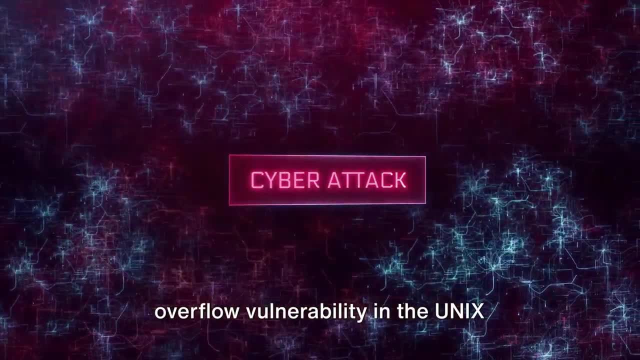 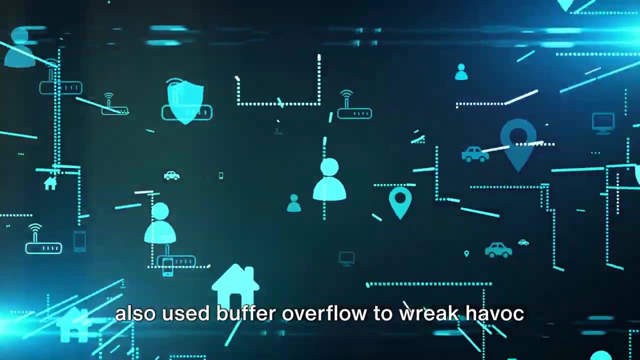 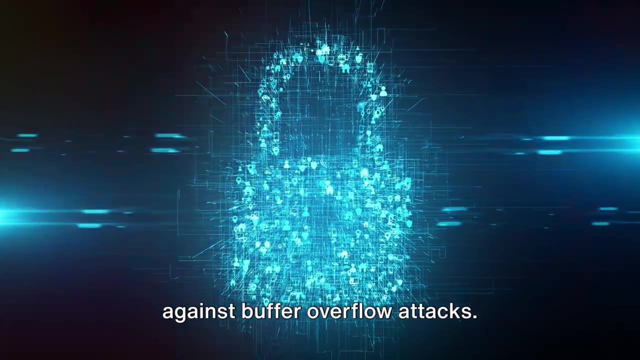 across the internet exploited a buffer overflow vulnerability in the unix systems fingered program. the infamous code red and slammer worms also used buffer overflow to wreak havoc on the internet. but it's not all doom and gloom. we covered various methods to guard against buffer overflow attacks. 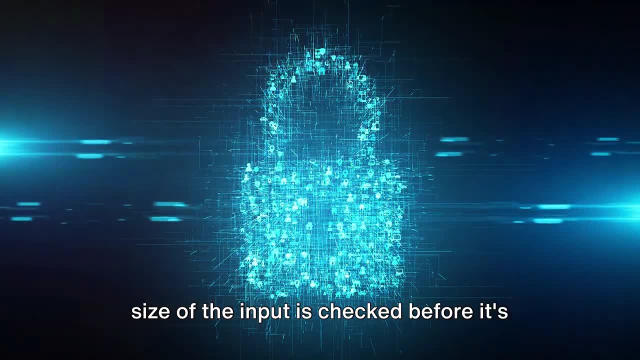 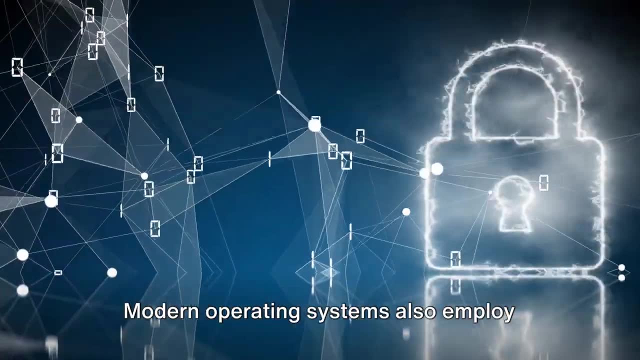 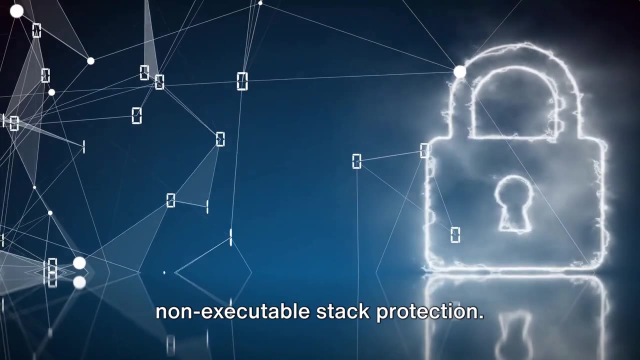 these include range checking, where the size of the input is checked before it's processed, and the use of secure coding practices that prioritize data input validation. modern operating systems also employ various security measures, such as address space layout randomization and non-executable stack protection. the future of buffer overflow. 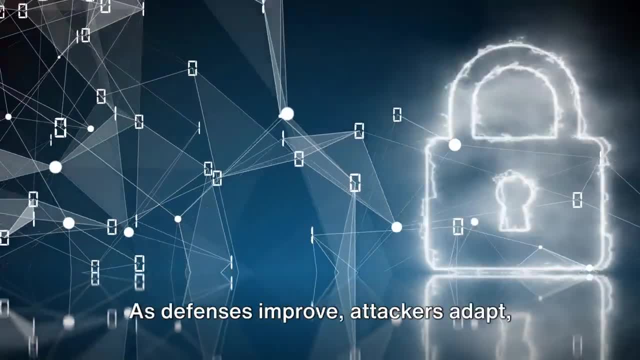 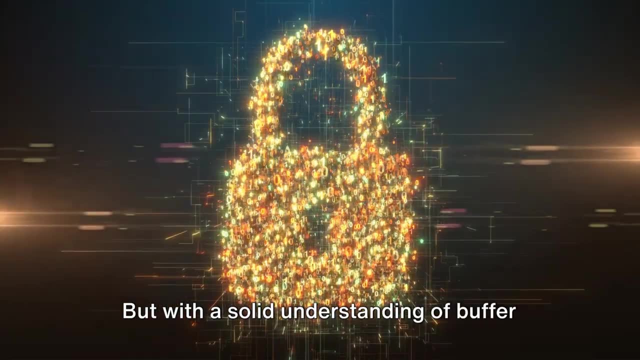 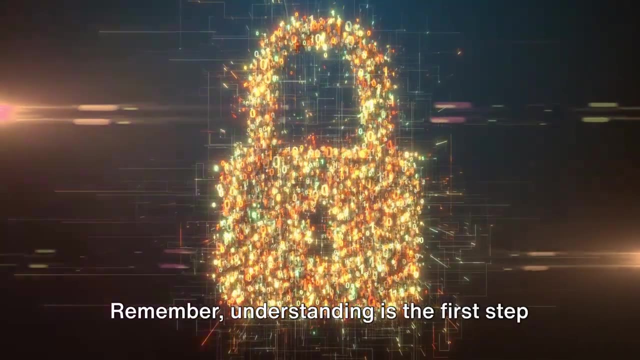 like any cyber security issue is a continuous gap of cat and mouse. as defenses improve, attackers adapt, finding new ways to exploit vulnerabilities. but with a solid understanding of buffer overflow we can anticipate potential threats and take preventative measures. remember, understanding is the first step to prevention, so let's keep our 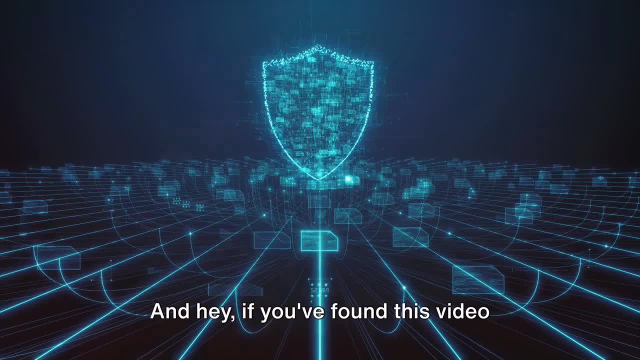 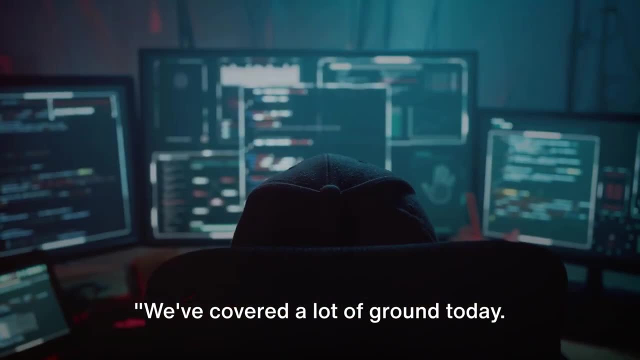 knowledge sharp and our systems secure. and hey, if you found this video helpful, don't forget to like, share and subscribe to my youtube channel. stay safe out there. we've covered a lot of ground today, from the real-life drama that unfolds with buffer overflow incidents to the intricate 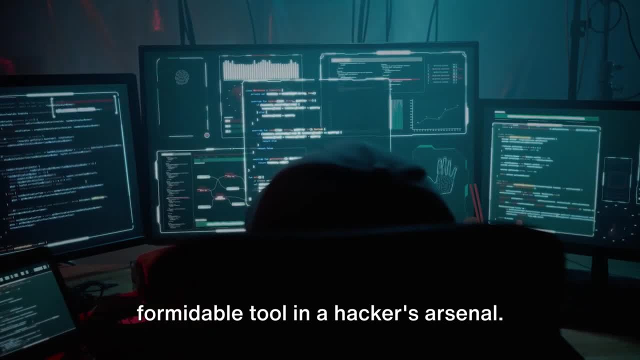 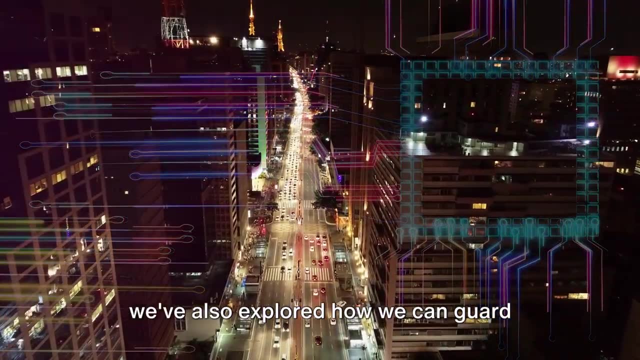 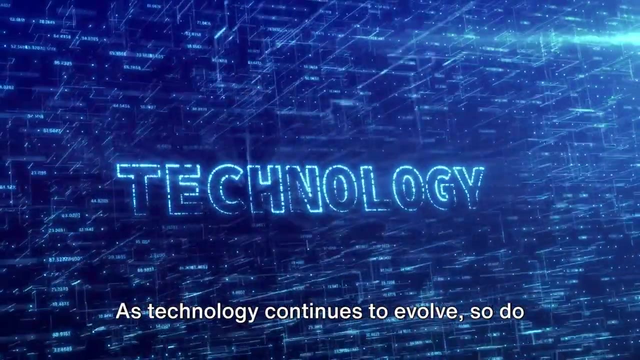 mechanics that make it a formidable tool in a hacker's arsenal. we've delved into some famous incidents that shook the world of cyber security, and we've also explored how we can guard against such attacks. let's not forget the future of buffer overflow, as technology continues to evolve. 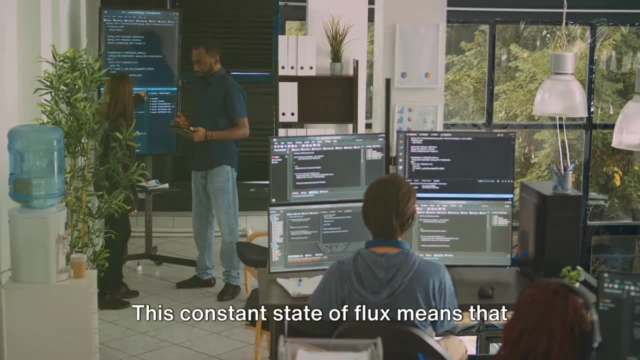 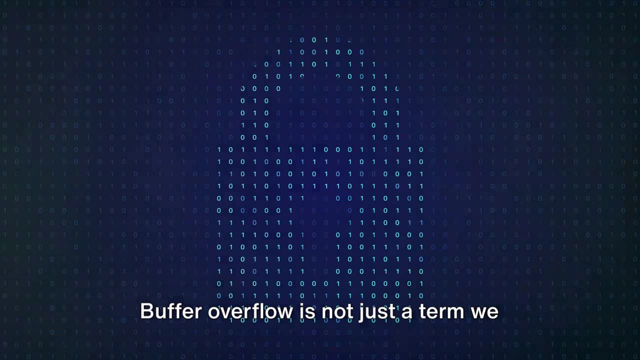 so do the threats we face. this constant state of flux means that our understanding of buffer overflows will continue to evolve. as technology continues to evolve, so do the threats we face. this constant state of flux means that our understanding of buffer overflow and cyber security in general needs to be dynamic. buffer overflow is not just a term. we